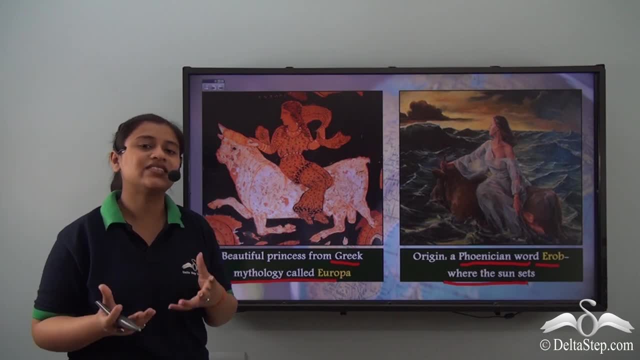 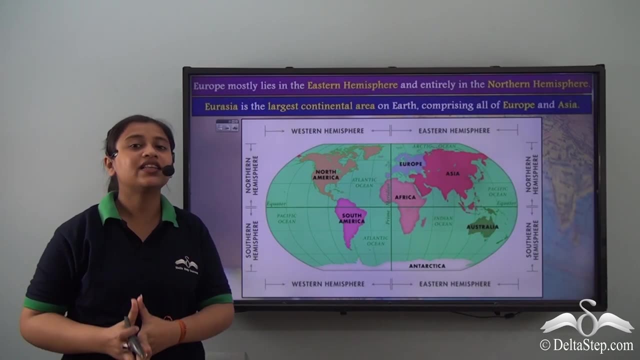 the two important origins from where it derives its name. So, as I just mentioned a while ago, that it is not in the western hemisphere but in the eastern hemisphere. So now let's actually locate Europe as a continent. So this is a world map showing different hemispheres. 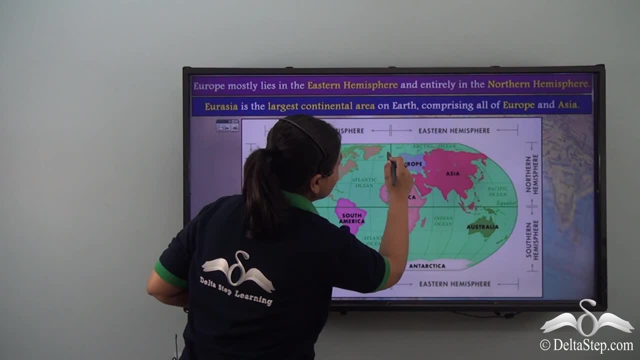 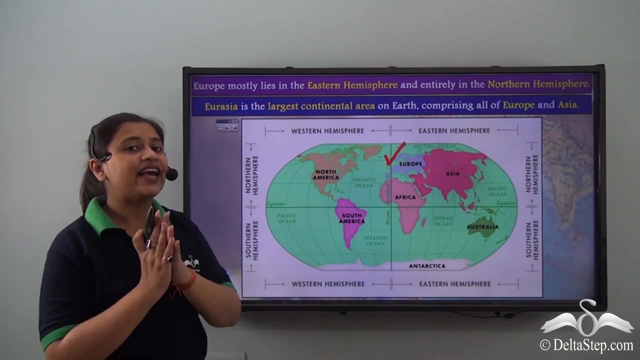 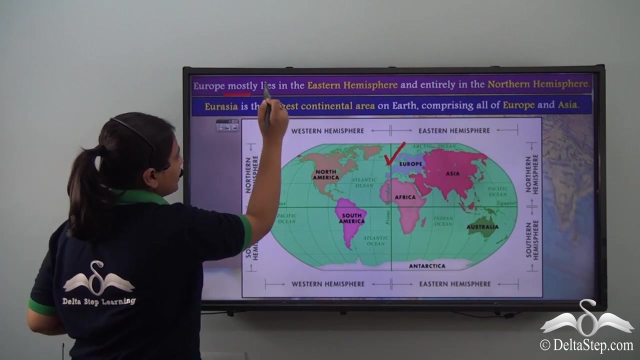 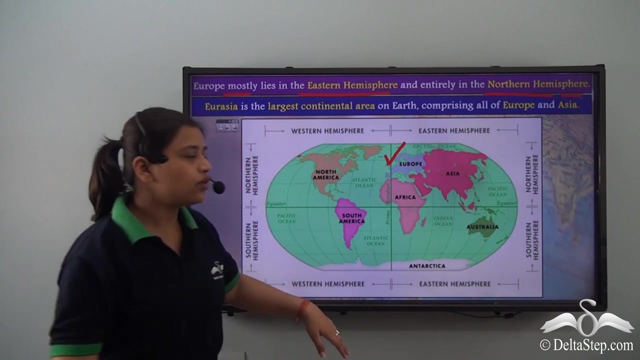 of the world. So you see, Europe right here is located almost on the eastern part and entirely on the northern hemisphere. So we can say that Europe mostly lies in the eastern hemisphere and entirely in the northern hemisphere, So we can say that it is a northeastern continent. Other 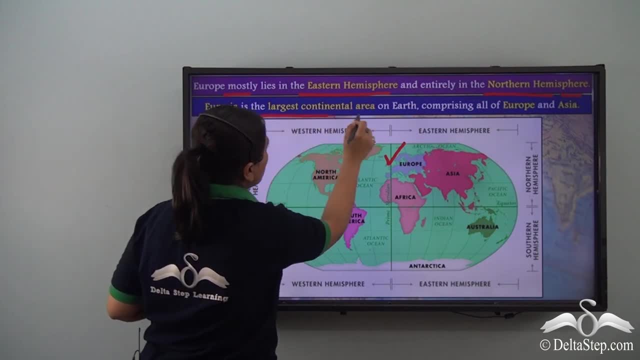 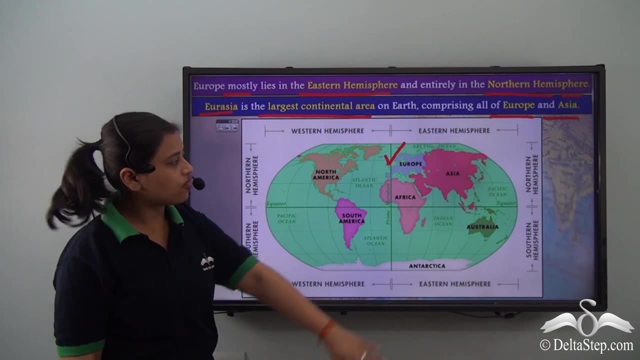 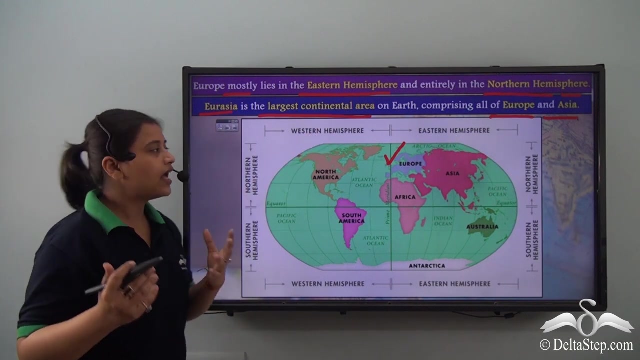 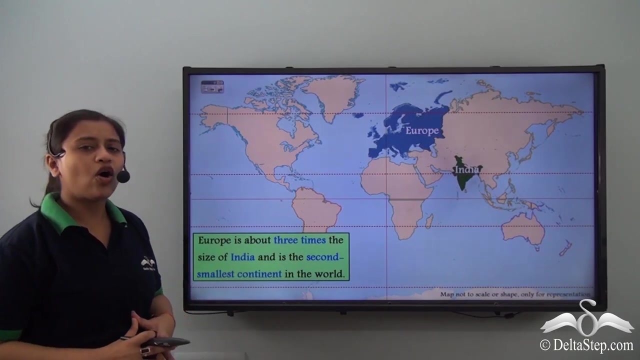 than that, Eurasia is the largest continental area on earth, comprising of Europe and Asia. So the continent of Europe and Asia together make up the largest continental area on earth. that is Eurasia. So now that we know that Europe lies almost in the eastern hemisphere and entirely in 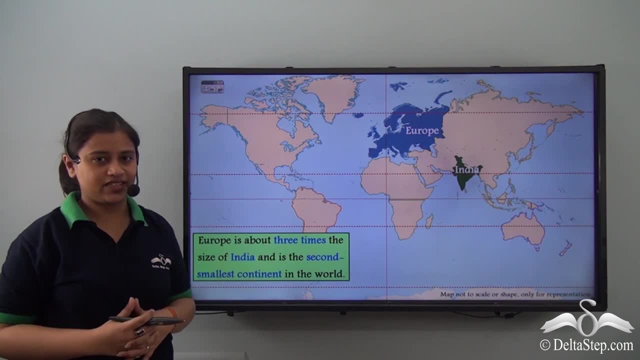 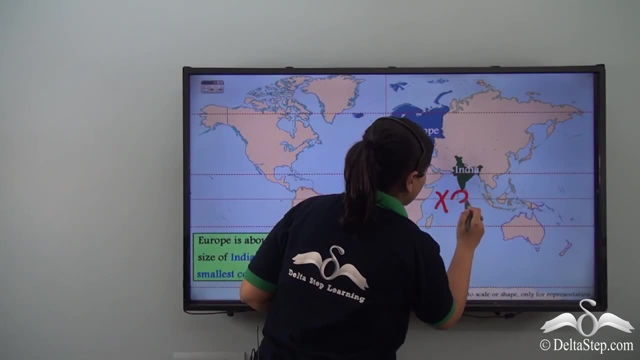 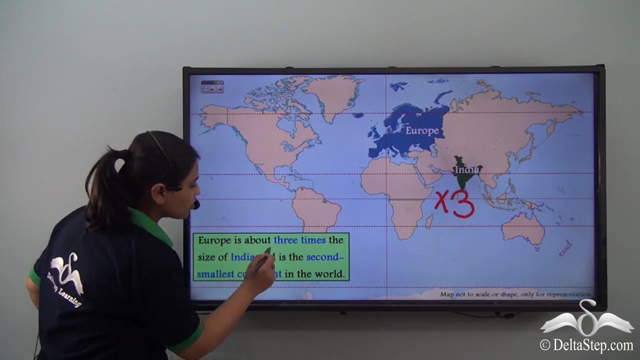 the northern hemisphere And if we conquer Europe, like the actor in the movie Let's, Let's talk about the size of the continent. Well, talking about the size of the continent, Europe is three times the size of India. So Europe is about three times the size of India. 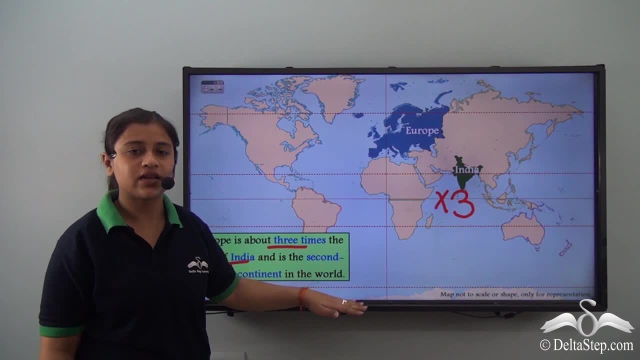 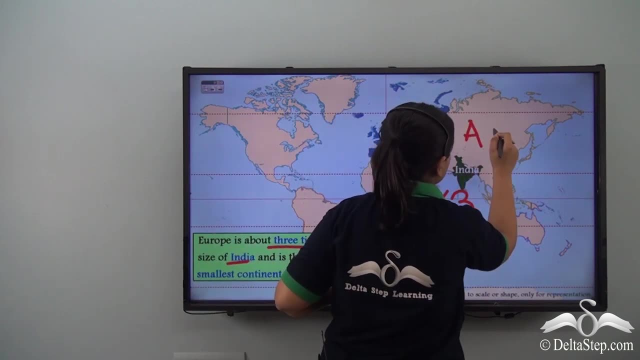 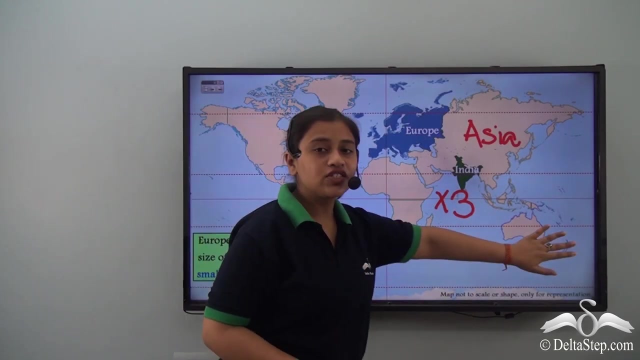 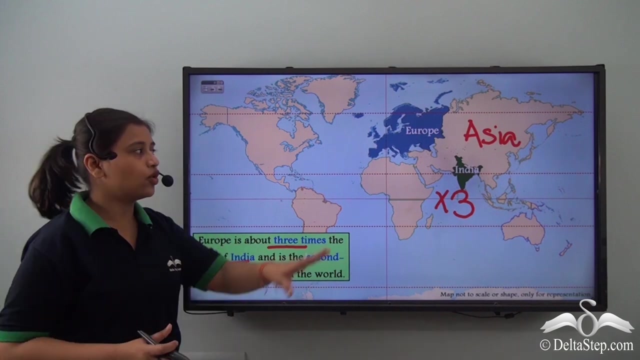 and is the second smallest continent in the world. So from this world map, we can see that the largest continent is Asia. The smallest continent on the map, as we can see, is Australia, and Europe is the second smallest continent in the world. So now we know the location. 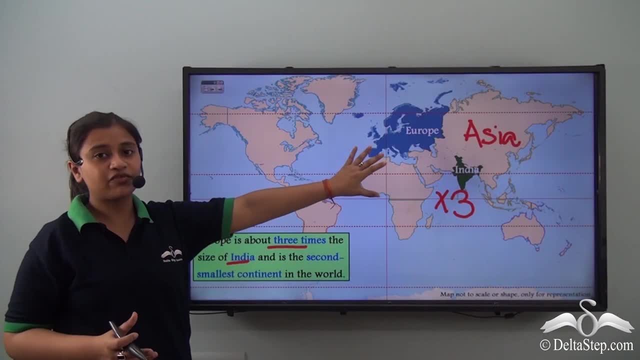 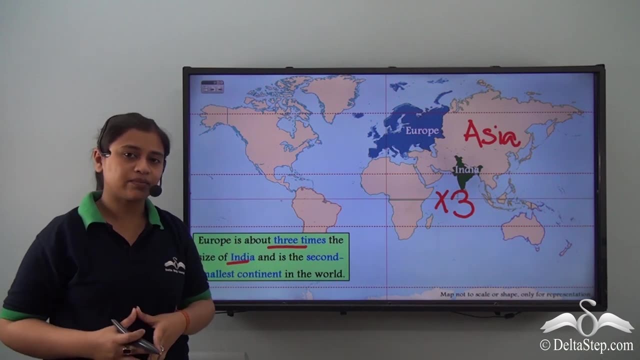 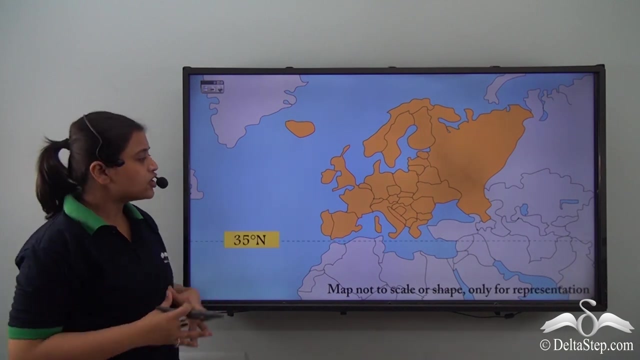 of Europe, a good idea of the size of Europe, which is three times the size of India, and it is the second smallest continent in the world. Now let us look at the map of Europe again. So we see that Europe lies in the temperate. 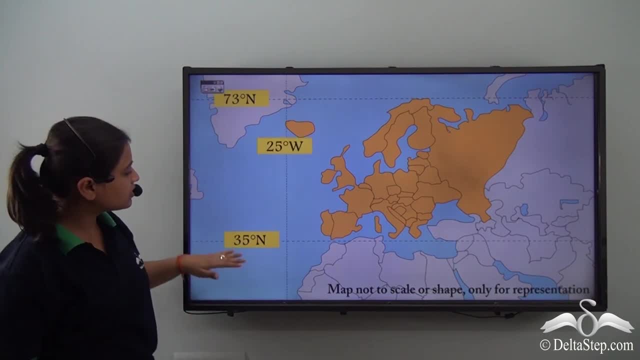 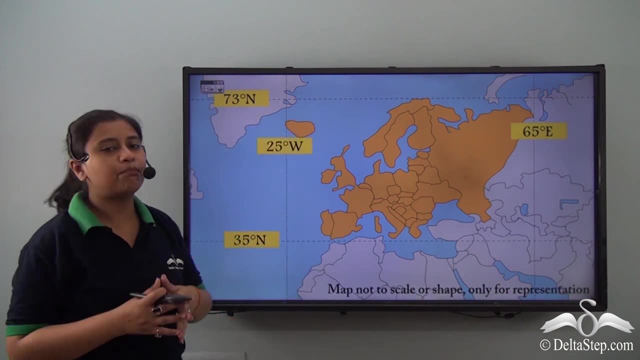 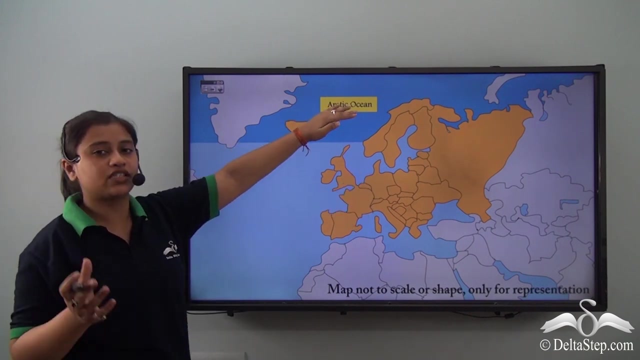 zone that is between 73 degree north to 35 degree north and between 25 degree west to 65 degree east. Now let's talk about the boundaries. Well, to talk about the boundaries, Europe is surrounded by Arctic Ocean to its north, then we have Atlantic Ocean to its south. 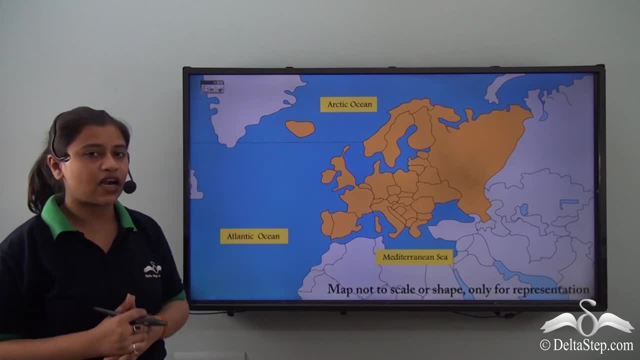 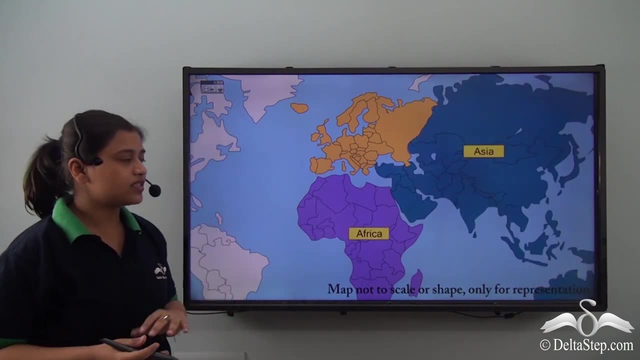 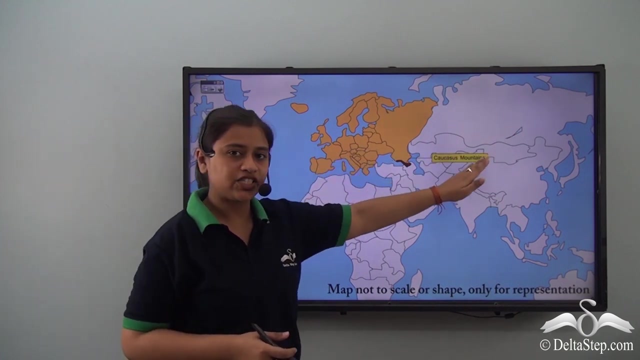 to its west and Mediterranean Sea to its south. So it is covered by three water bodies on three sides. Well, its immediate neighbours are Asia and Africa. Other than that, Europe is separated from Asia by these physical features: Ural Mountains, Caucasus Mountains, Black 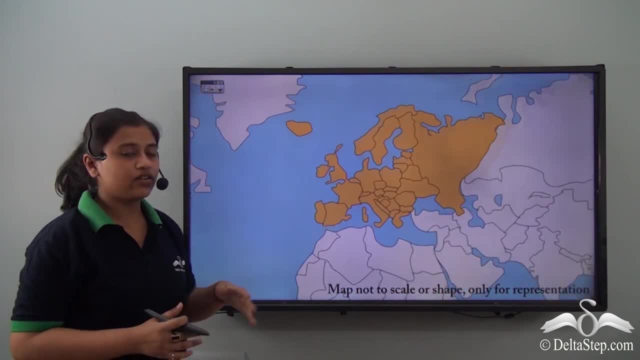 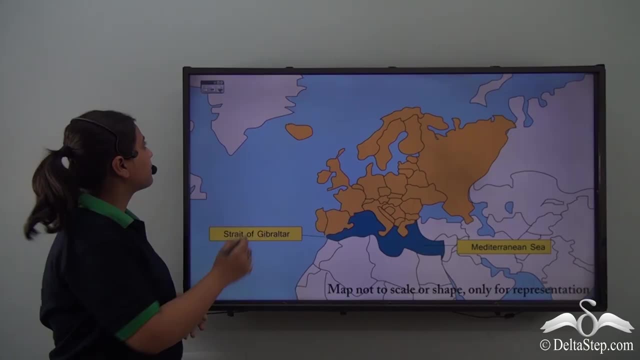 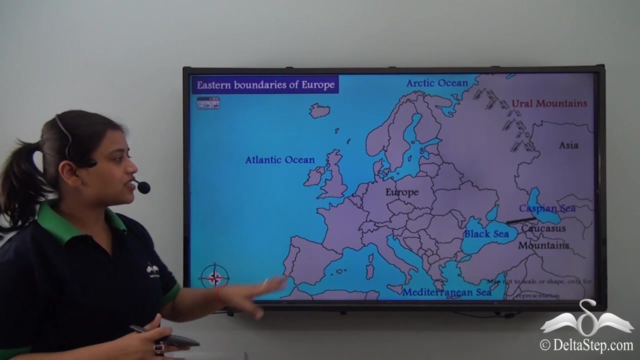 Sea and Caspian Sea. On this side, or on the southern part, it is separated from the Arctic Ocean, from Africa, by the Strait of Gibraltar in the Mediterranean Sea. Now let us look at the eastern boundaries of Europe again. that separates the continent of Europe from 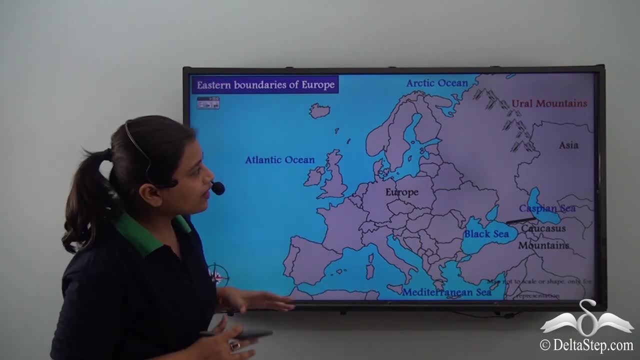 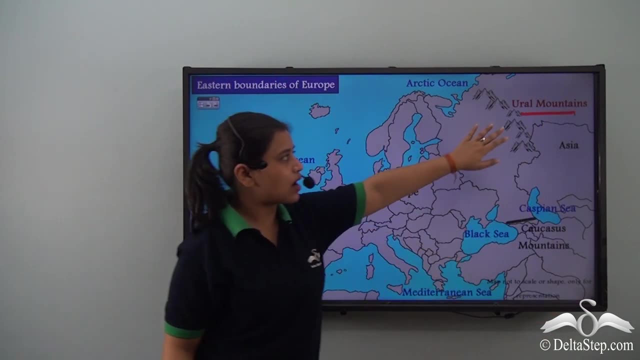 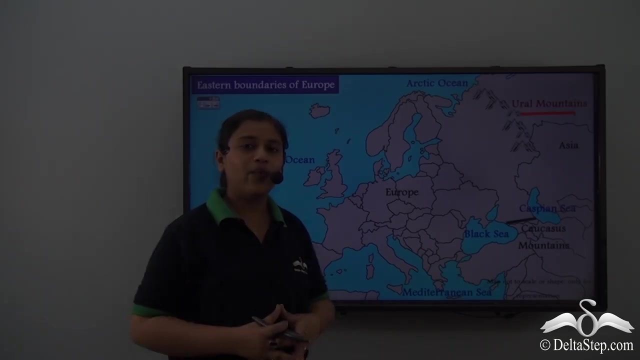 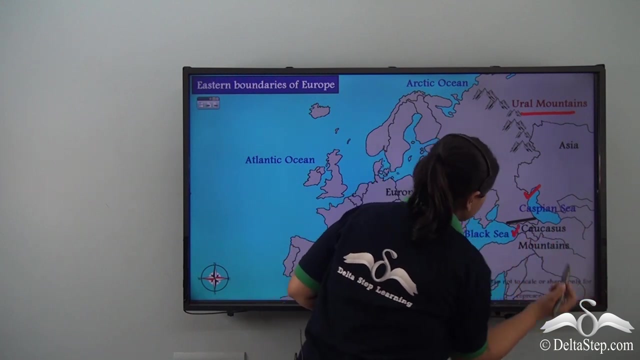 the continent of Asia. So on the very northeastern part we have the Ural Mountains. Now you see that the Ural Mountains in the northeastern part separates or act as a boundary between Europe and Asia, While in the southeastern part we have the Caspian Sea, the Caucasus Mountains and the. 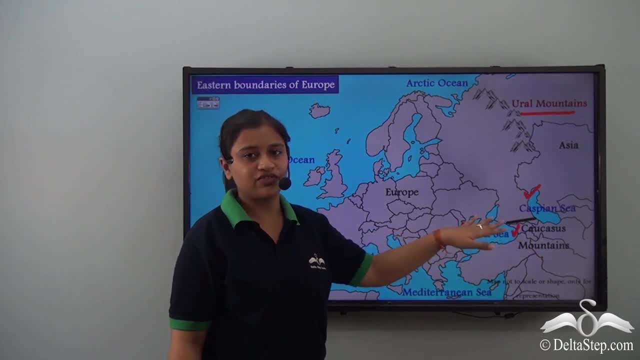 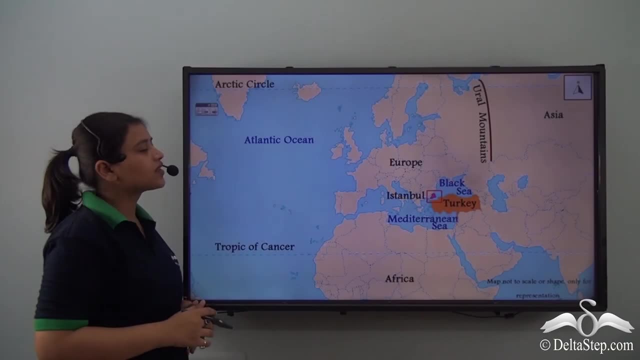 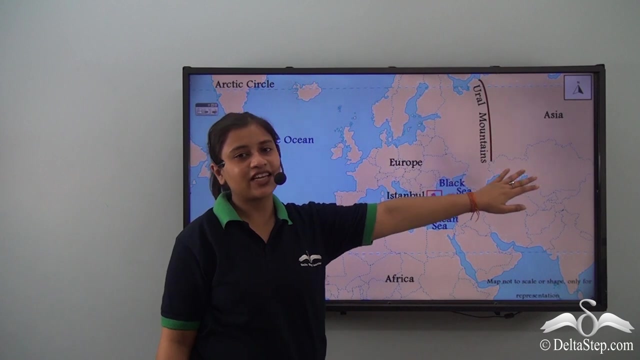 Black Sea. So these in the southeastern part of Europe separate this continent of Europe from Asia. However, there's a small region that connects the continent of Europe to the continent of Asia. This small region is here near Istanbul. So this small region connects. this small region here to the continent of Asia, So it is called Justi because it contacts here to the Pakistan. So this smallこれは is the north east high trace which is called Eastu. So this is their location. should Tanda place, which is located in South east under У embankment. 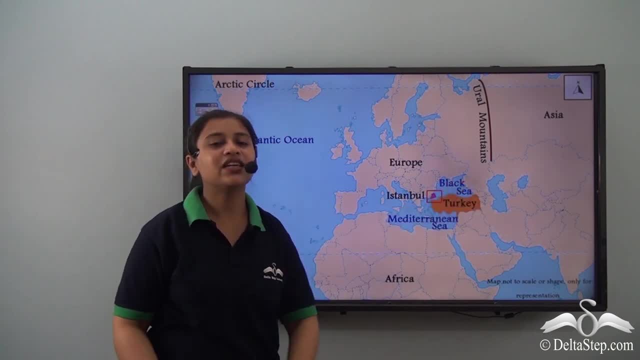 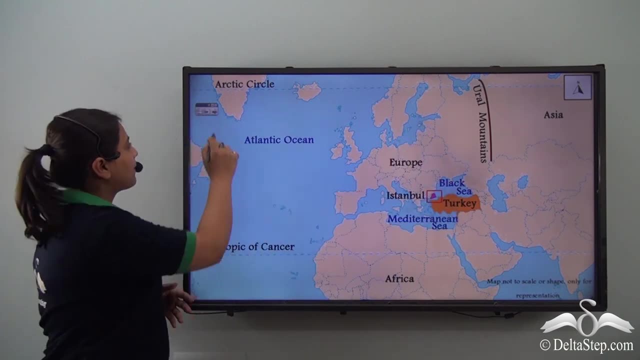 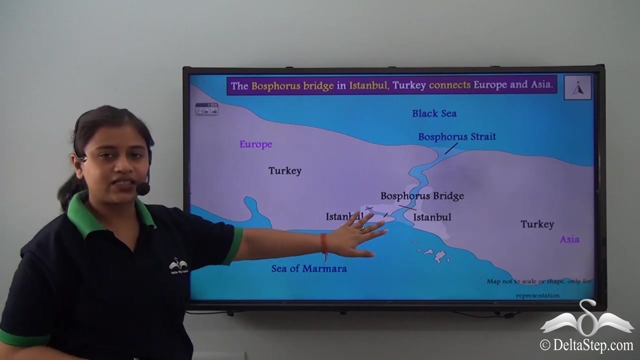 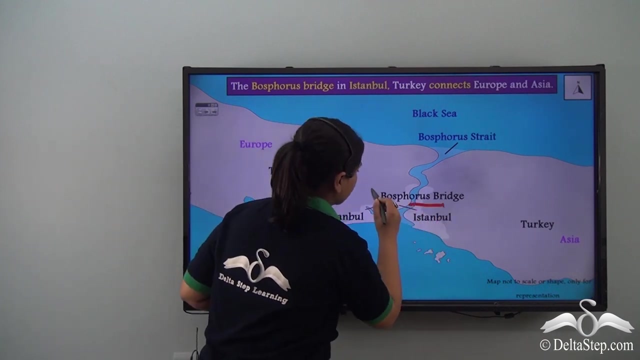 Istanbul and Turkey near the Black Sea. So let's have a zoomed in view of what exactly connects these two continents. So this is a zoomed in view where the European part of Istanbul is connected to the Asian part of Istanbul by the Bosphorus bridge. Yes, a very 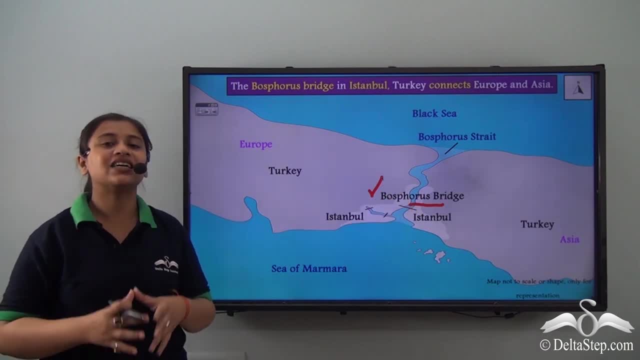 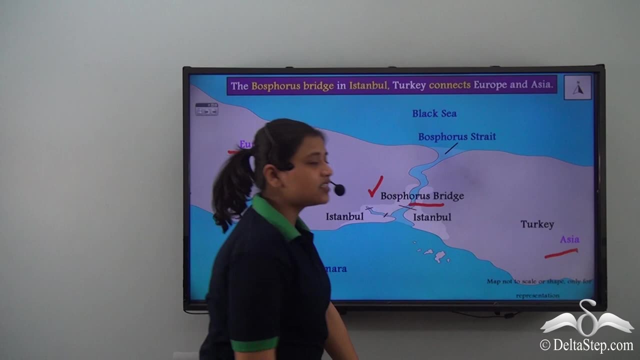 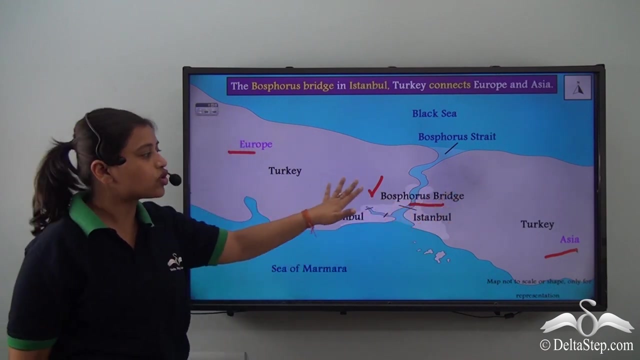 important bridge that can also be called as a connection between the continent of Europe and the continent of Asia in the southeastern part. So we see that the Bosphorus strait that separates the two continents here is contradicted by the Bosphorus bridge at the 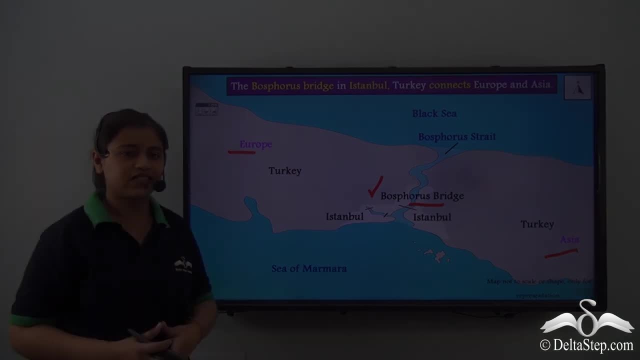 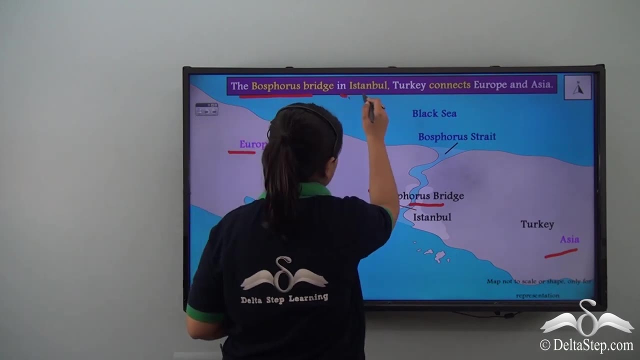 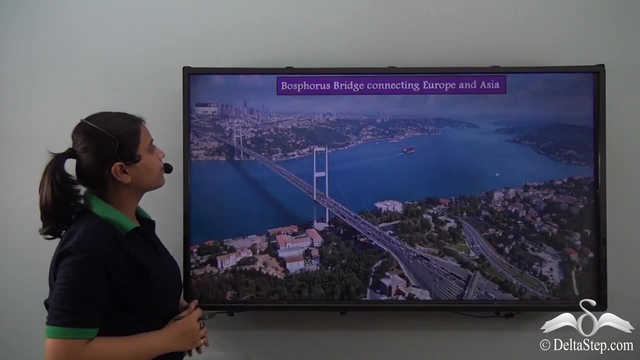 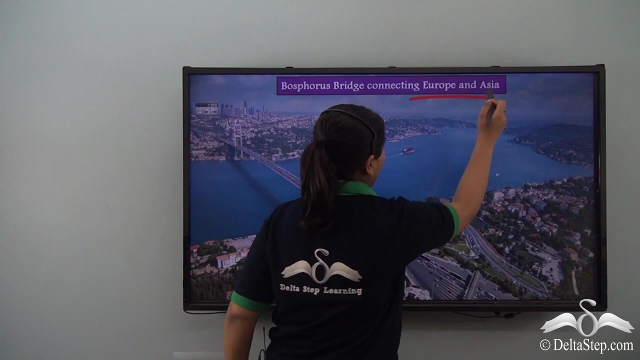 same place that connects these two continents. So we just understood that in the southeastern part of the continent, the Bosphorus bridge in Istanbul, that is, in Turkey, connects Europe and Asia. So this is a real image of the Bosphorus bridge connecting Europe and Asia. So, before moving on, could 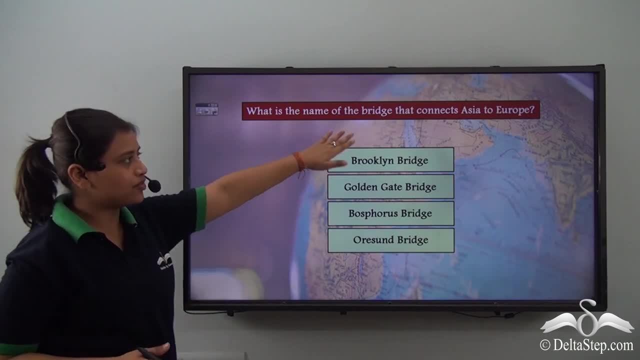 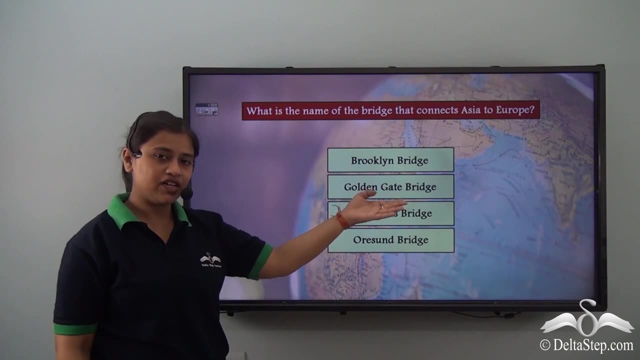 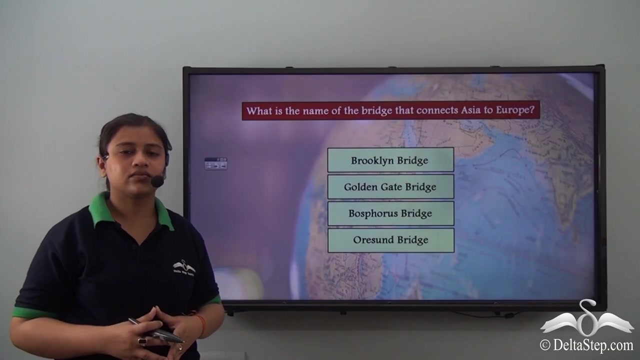 you help me answer this simple question. What is the name of the bridge that connects Asia to Europe? Is it the Brooklyn Bridge? Yes, the Brooklyn Bridge Bridge, or the Golden Gate Bridge, or the Bosphorus Bridge or the Orsund Bridge? Sit down, Yes, 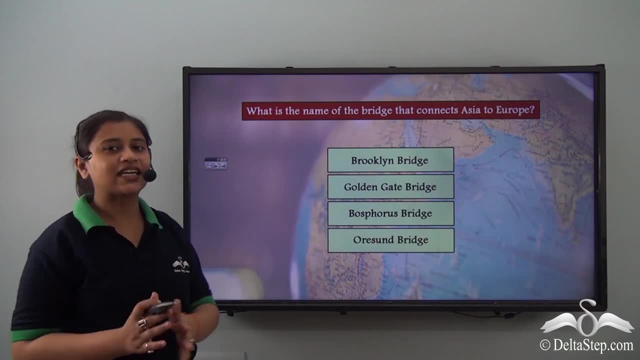 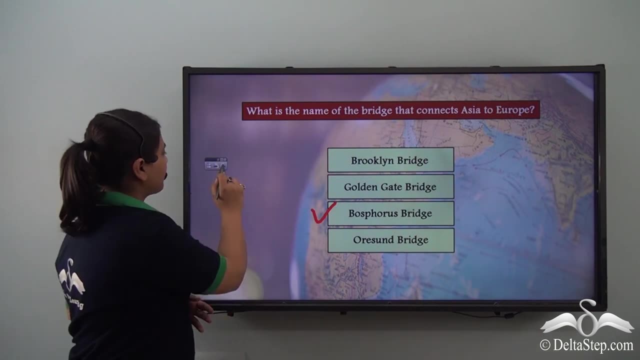 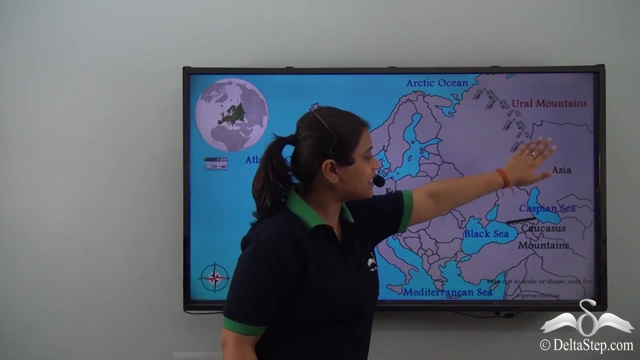 you have guessed it right that the Bosphorus Bridge connects Asia to Africa, So the right answer is the Bosphorus Bridge. So now that we have located the continent of Europe, we have learnt about the important eastern boundaries that separates Europe from Asia. We also learnt 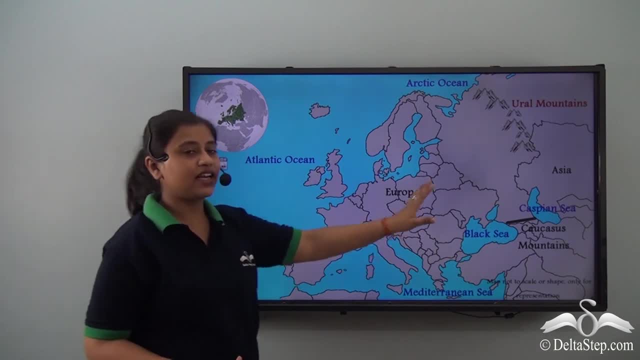 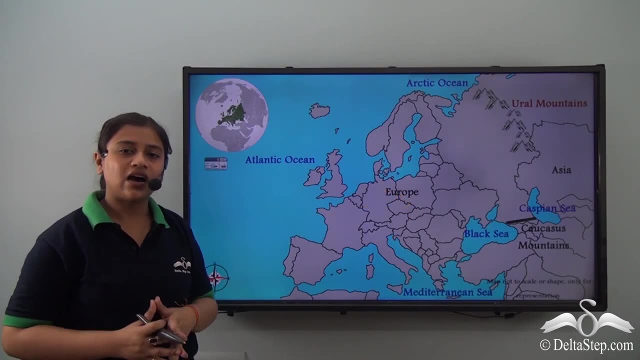 about the Bosphorus Bridge that connects Europe and Asia in the south eastern part, and we learnt about the European continent that surrounds the European continent on the western part, the northern part and the southern part respectively. So now let's have a look at the map of Europe. 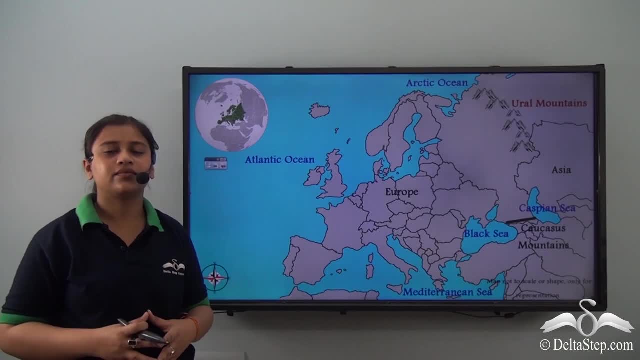 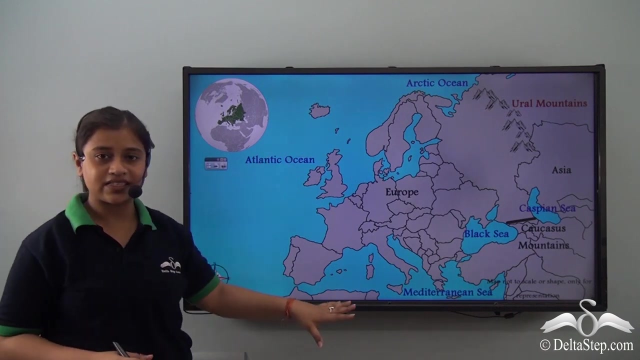 from a geographical perspective. So what do you observe about this physical feature of this particular continent? Is there something different or unique about it? So you can see that it is surrounded by water bodies on three sides, while it is connected to a main land on one side. Do we have a name for this physical feature? Yes, this physical feature is the. 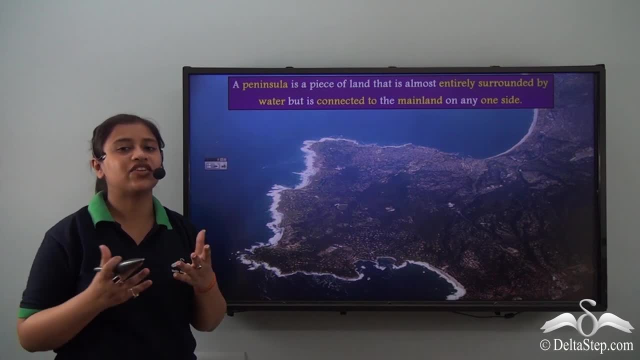 Bosphorus Bridge. The Bosphorus Bridge connects Asia to Africa. Yes, this physical feature connects Asia to Africa. Yes, this physical feature connects Asia to Africa. Yes, this physical feature is regarded or considered as a peninsula. So what exactly is a peninsula To define? 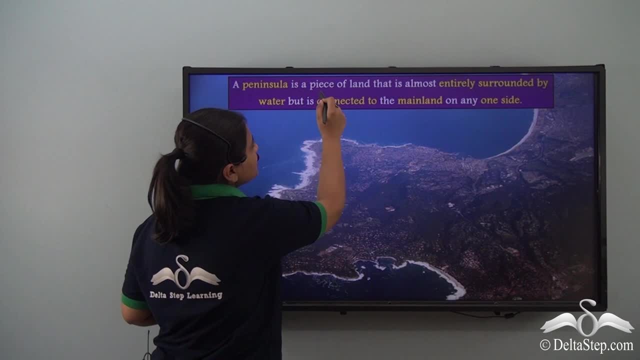 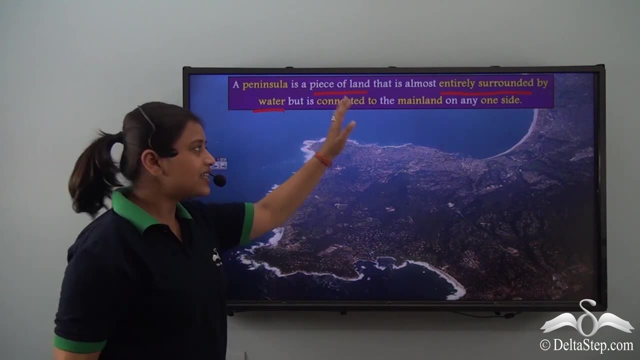 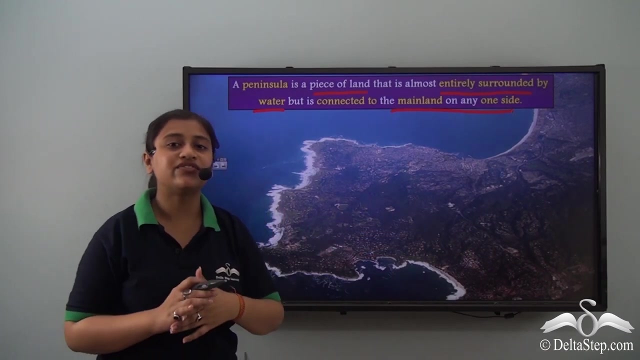 peninsula. we could say that a peninsula is a piece of land that is almost entirely surrounded by water but is connected to the main land on one side, Image here. So this image here also defines or helps us understand the definition of a peninsula. So we can see, so this piece. 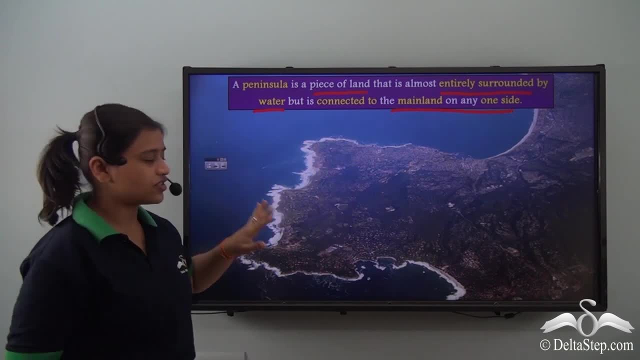 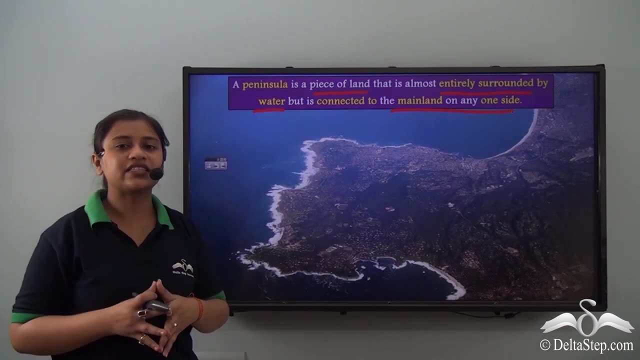 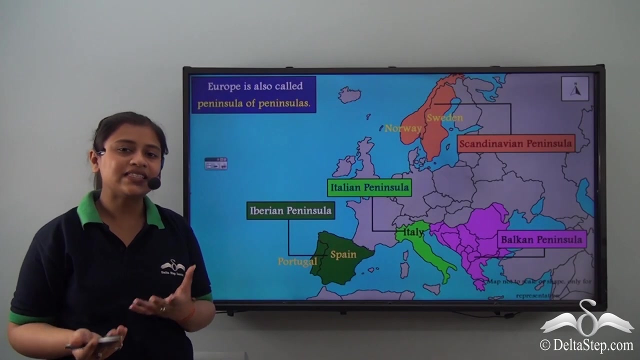 of land is surrounded by water bodies on three sides, while it is connected to a main land on one side. So this type of physical structure or feature is known as a peninsula. So we can now say that Europe is a peninsular continent. Other than that, it is not only a peninsula. 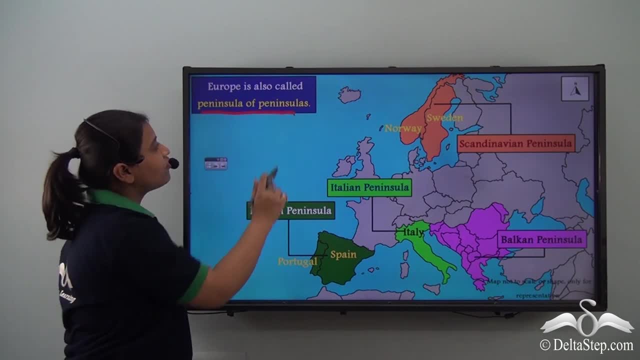 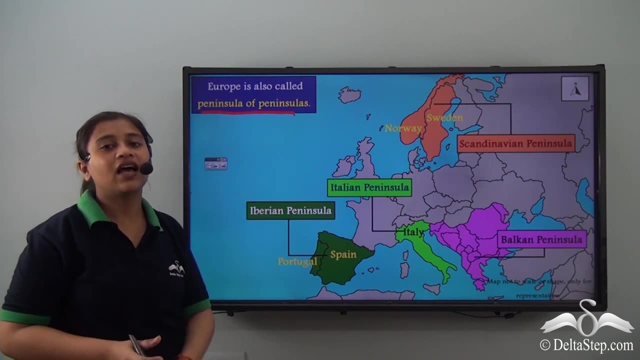 it is also known as a peninsula of peninsulas- Peninsulas- Wow, that's interesting. Why is it known as a peninsula of peninsulas? Because, being a peninsula, it has several smaller, other important peninsulas within itself. So you can see these. 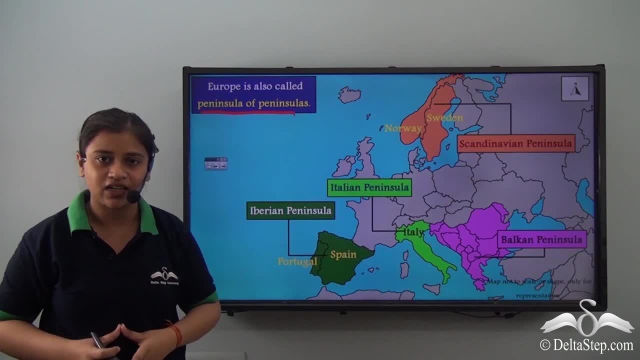 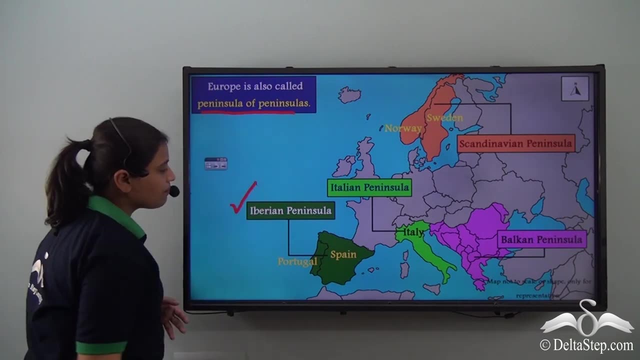 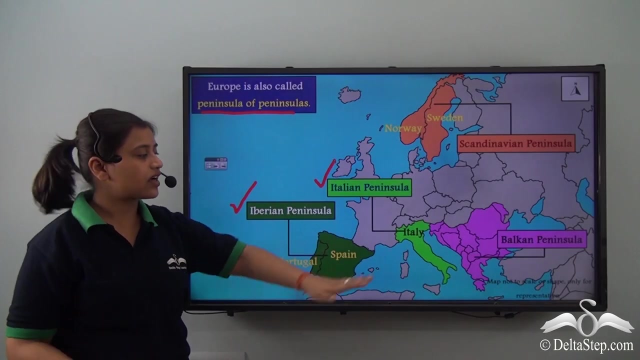 are some of the most important smaller peninsulas in Europe. Let's name them. So the major peninsulas within Europe are the Iberian Peninsula, which covers the countries of Portugal and Spain. Then we have the Italian Peninsula, covering the country of Italy. Then we have 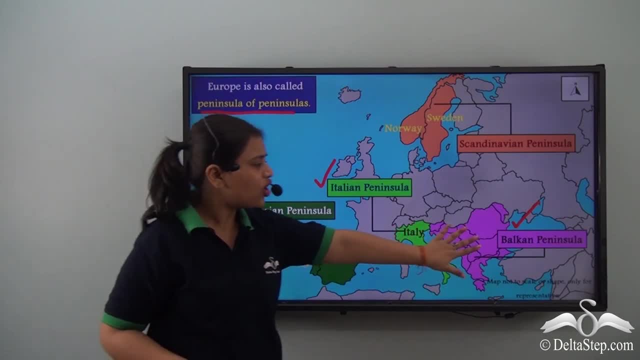 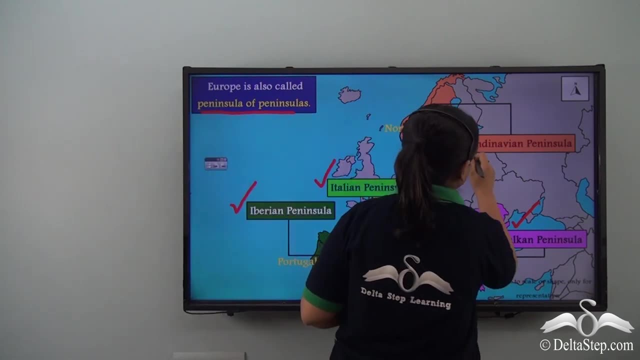 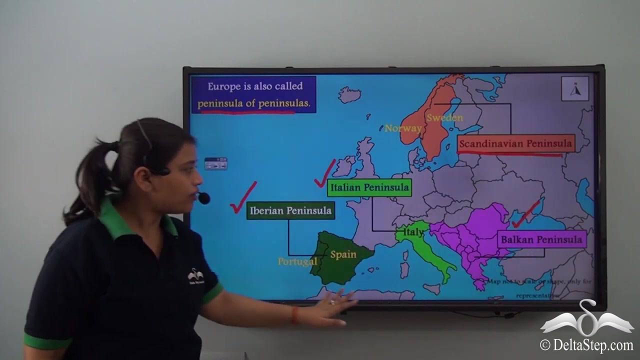 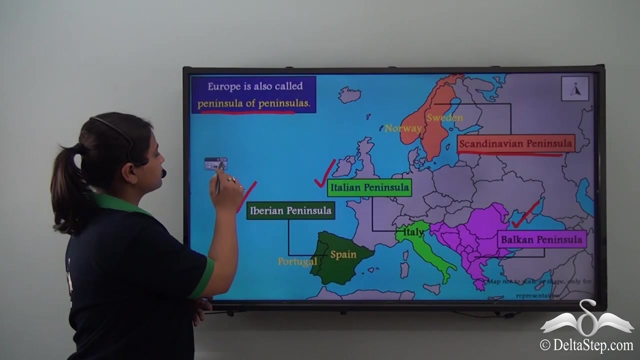 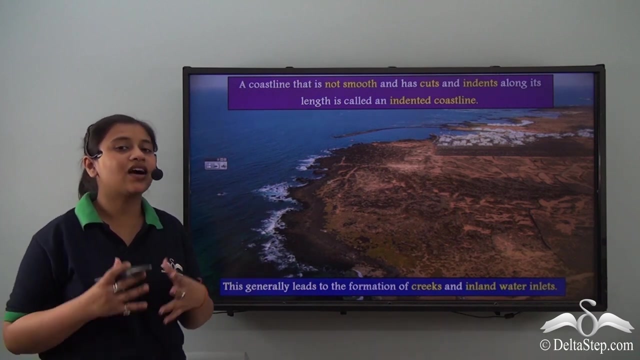 the Balkan Peninsula, which covers a lot of countries in the southern part of the continent, And then we finally have the Scandinavian Peninsula that comprises of Norway and Sweden. So these four peninsulas are some of the major peninsulas of Europe. So now we know that Europe is a peninsula, but other than that there is another very 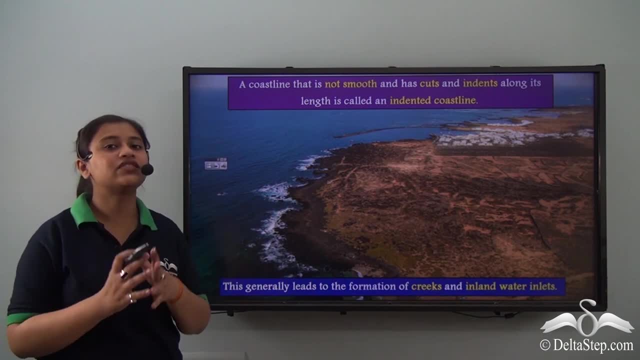 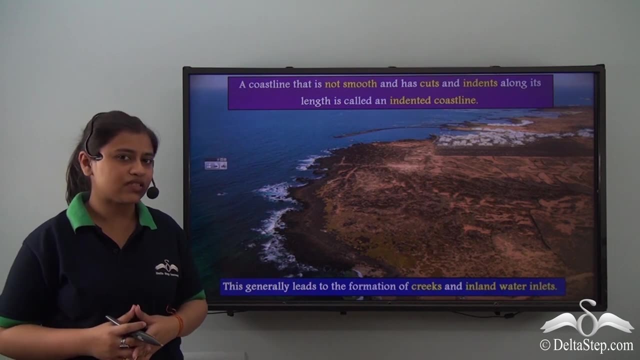 special feature to its physical structure or physical appearance. So if you have been noticing carefully the map of Europe, then you must have noticed that the coastline of Europe is not smooth. right, There are many cuts and indents, So such a coastline is. 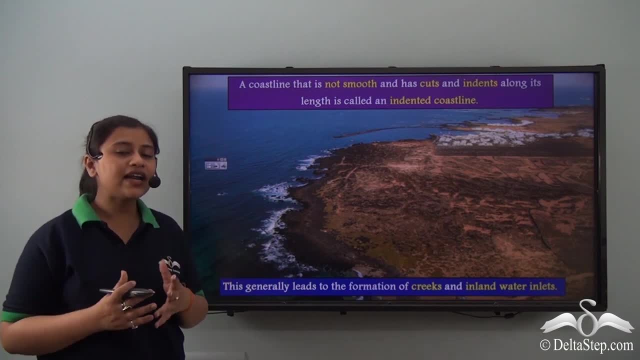 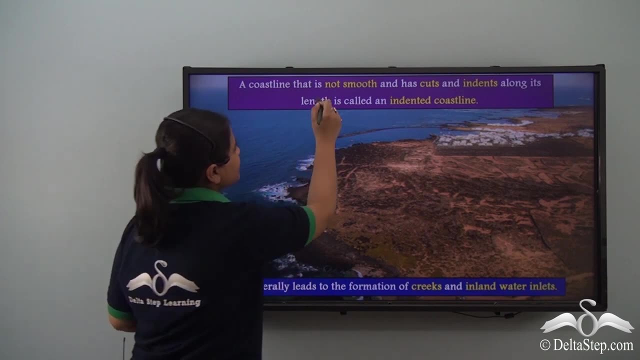 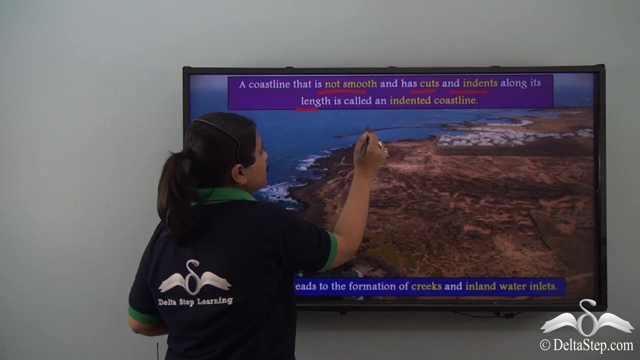 called an Indented Coastline. So to define what is indented coastline, let's look at this particular definition. So a coastline that is not smooth and has cuts and indents along its length is called an Indented Coastline. So from this image also you can understand. 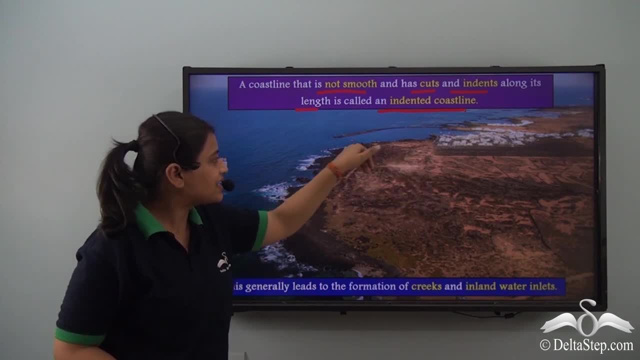 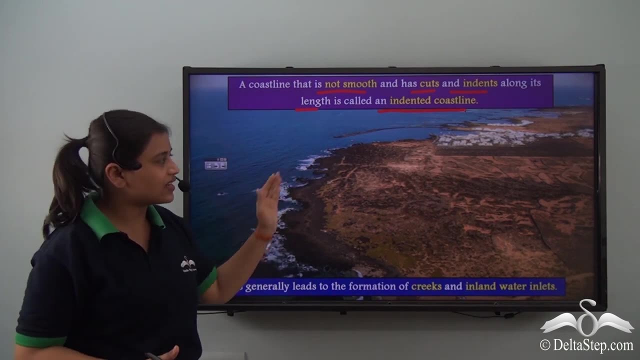 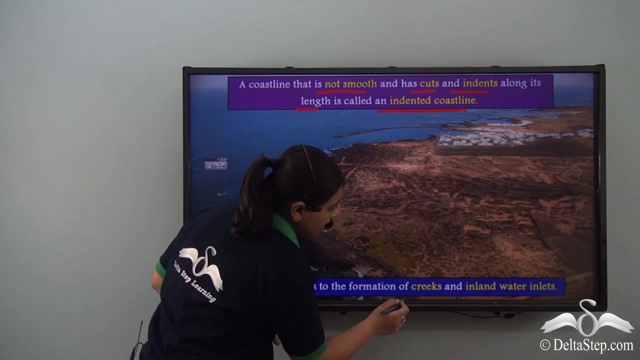 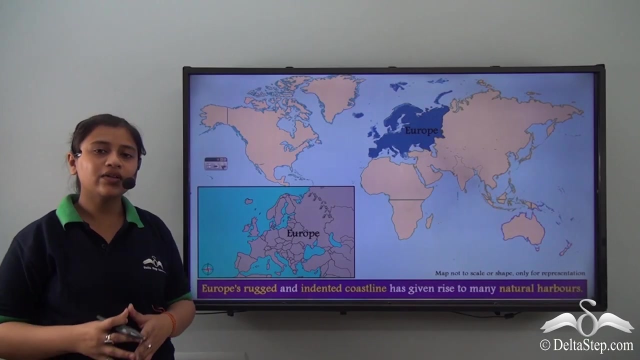 that this particular landmass has an Indented Coastline, as the coastline of Europe. The coastline is not smooth and there are many cuts and indents on the coastline. Such indented coastlines give rise to the formation of creeks and inland water inlets. right Now, let us 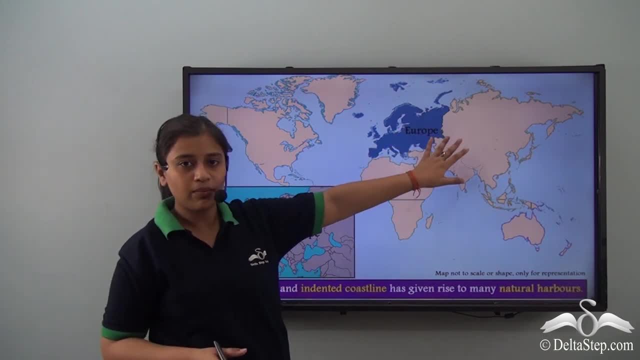 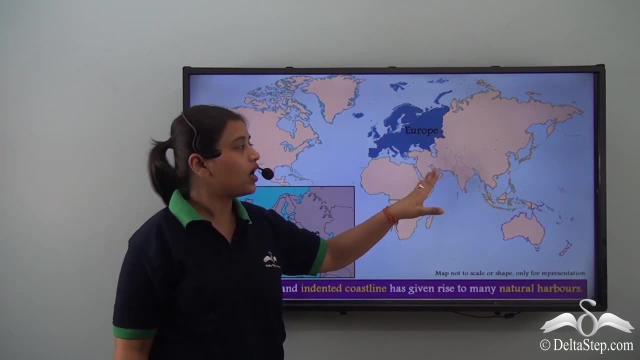 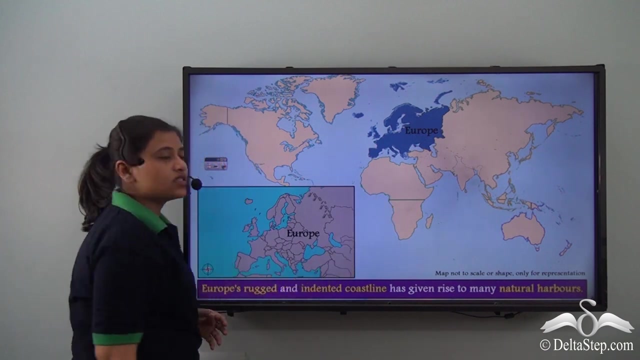 look at the map or the continent of Europe on this world map. So you see, in comparison to other continents on the world map, Europe has the most uneven coastline. So, for example, the continent of Africa. So you see that the coastline is much more smoother as compared. 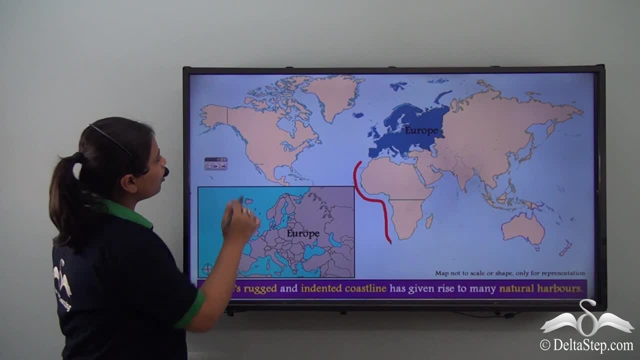 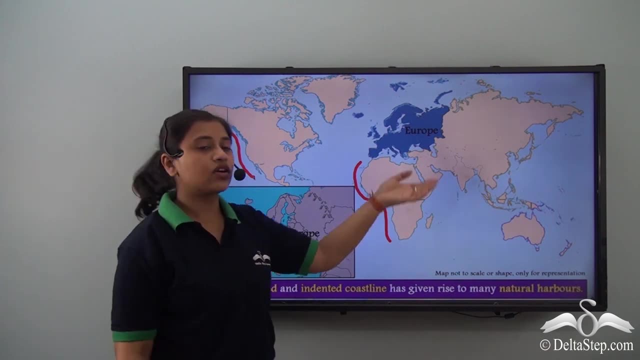 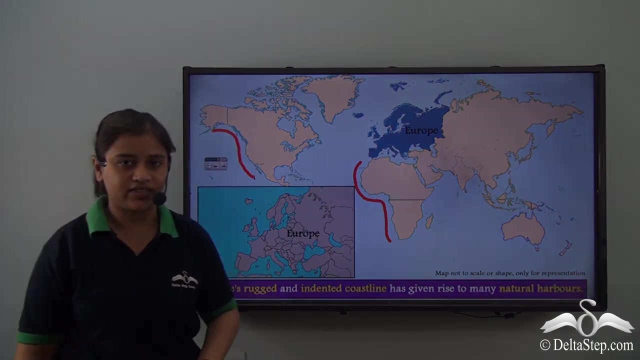 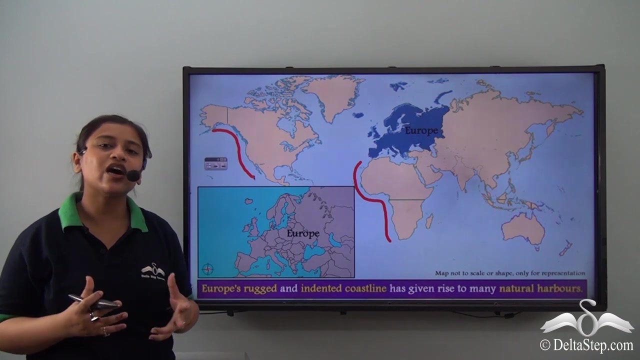 to that of Europe, Similarly that of North America. The coastline is much more smoother and gentle as compared to the continent of Europe, So we can say that Europe has a rugged and uneven coastline. However, this indented coastline has given the continent an economical benefit. How is that So Europe's rugged and indented coastline? 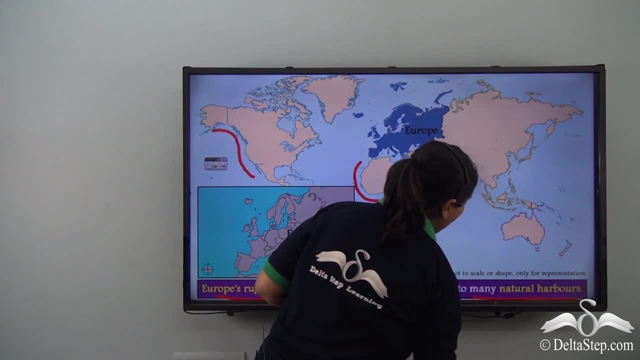 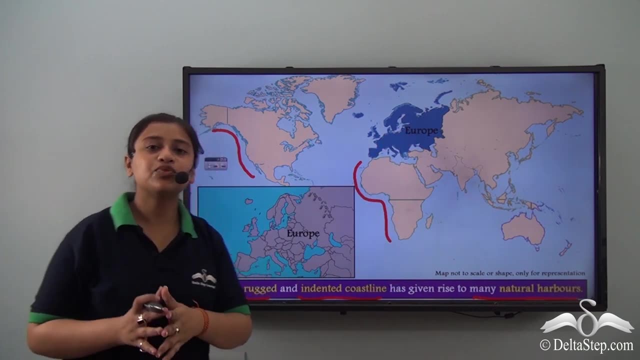 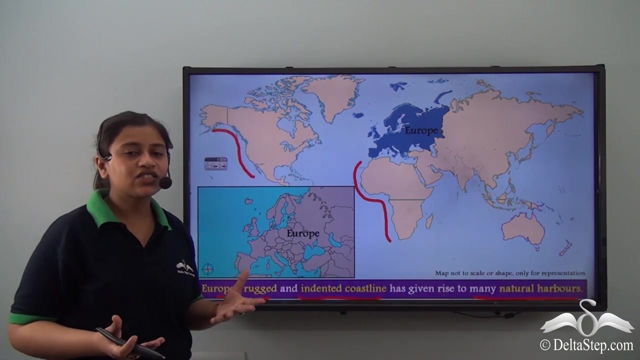 has given rise to many natural harbours. Well, so the indented coastline of Europe has proven to be an advantage by giving rise to many natural harbours. Now, why is it an advantage? Are natural harbours really important? Before understanding that, let us understand what. 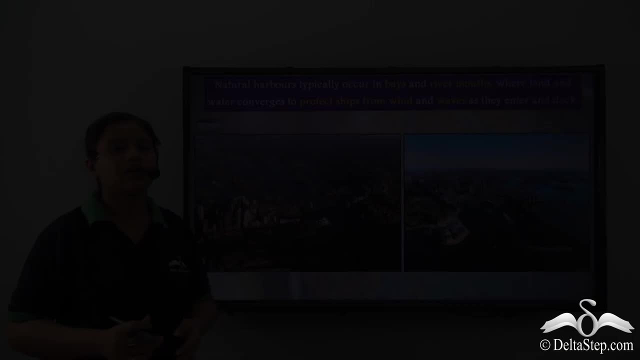 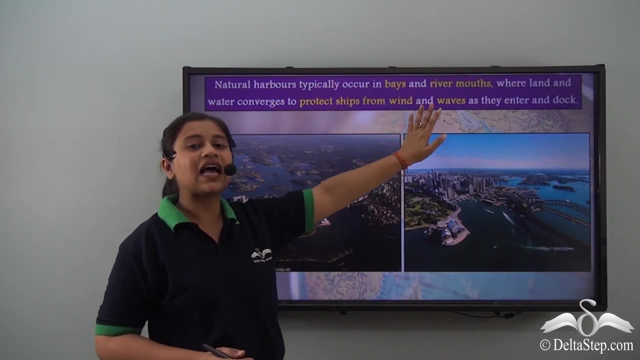 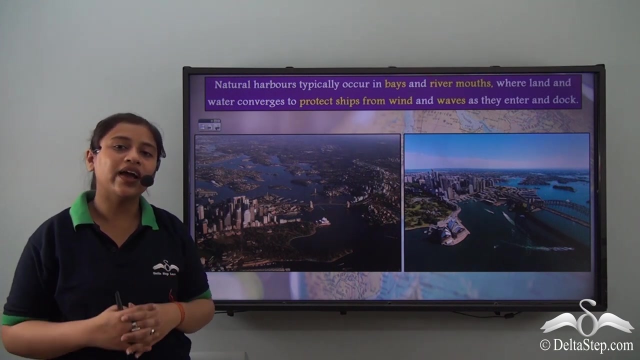 exactly are natural harbours. So, to define natural harbours, we could say that natural harbours typically occur in bays and river mouths. So bays are round shaped river mouths. And what are river mouths? Well, where the rivers enter into larger water bodies, right. So they occur typically in bays and 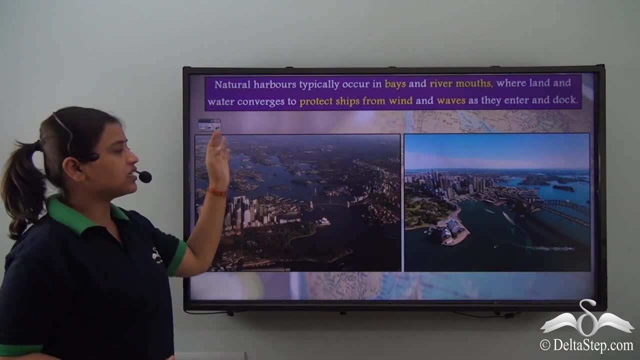 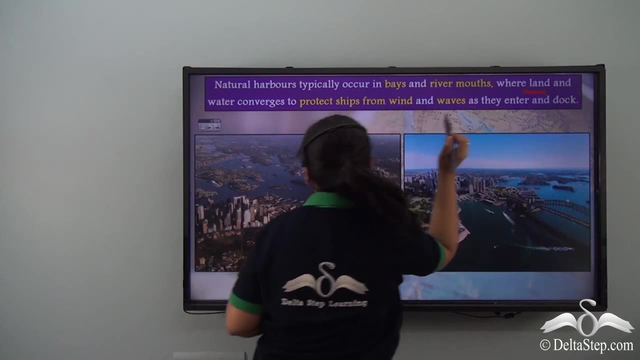 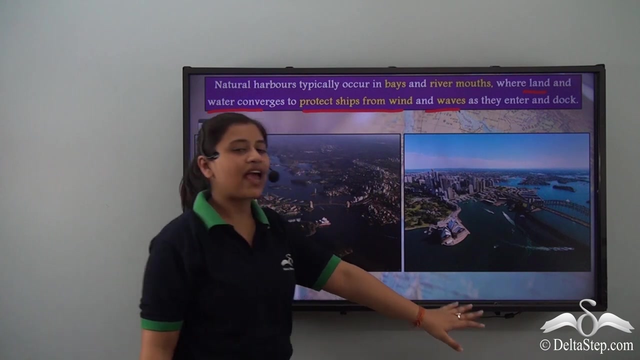 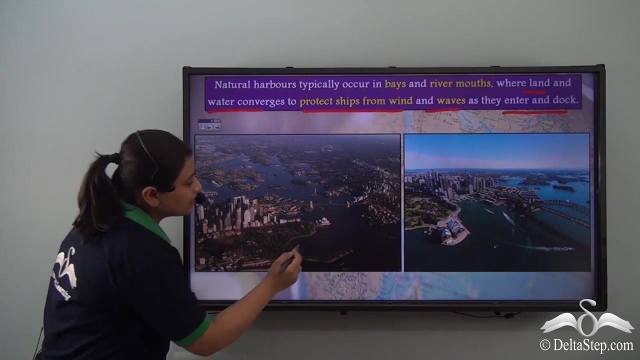 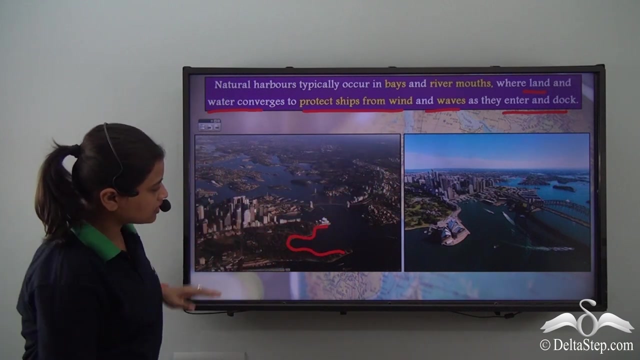 river mouths, where the land and water converges to protect the ships. So here the land and the water has converged to protect the ships from wind and waves as they enter these natural harbours and dock. So on this particular picture, you can see that this area here is like an enclosure where the land and water 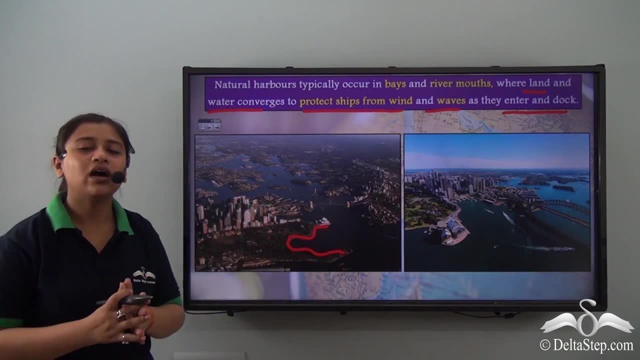 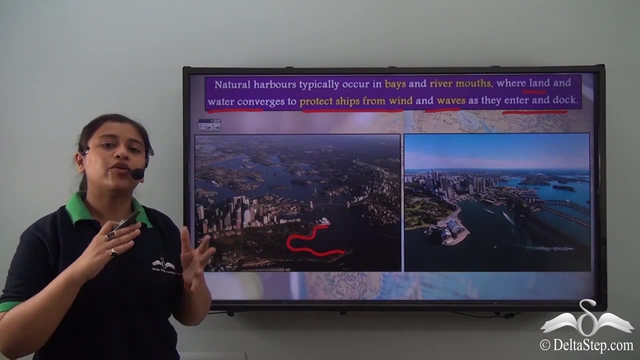 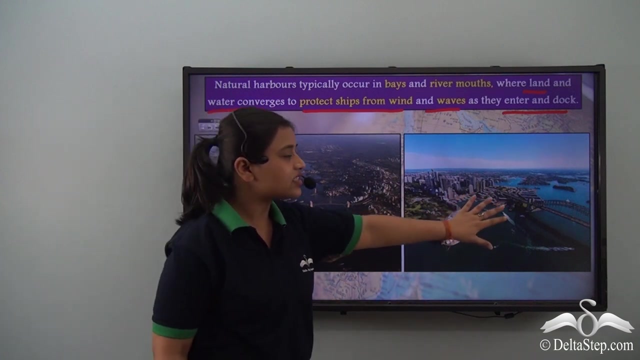 see, the land and water has nearly converged to form a protected area for the ships. So this particular convergence actually helps the ships or protects the ships from winds and waves as they enter and dock. So, as you can see that this is a zoomed in picture of 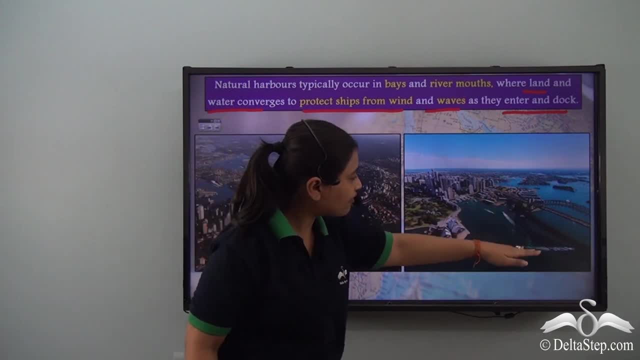 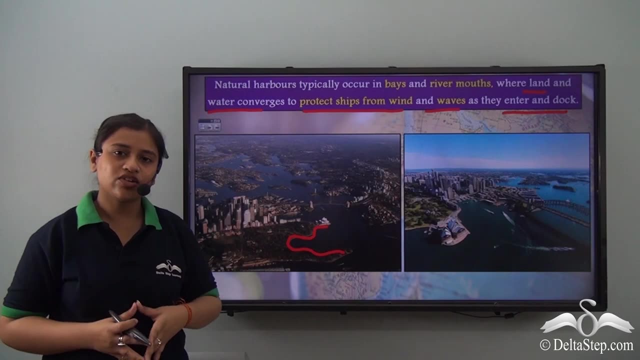 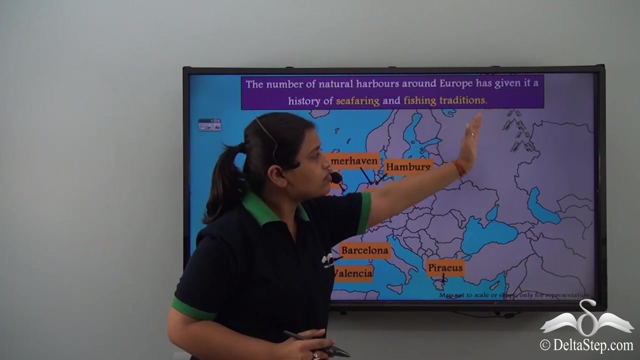 this particular area. So you see that the ships have entered and docked right here and this is an example of natural harbour. Just so you know, this particular image is of the largest natural harbour in the world, which is in Sweden. Now, the number of natural harbours around Europe has given. 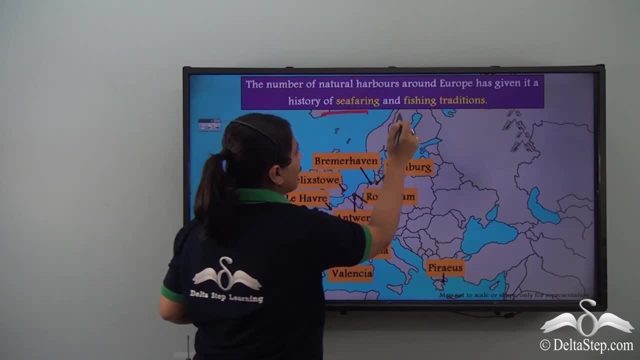 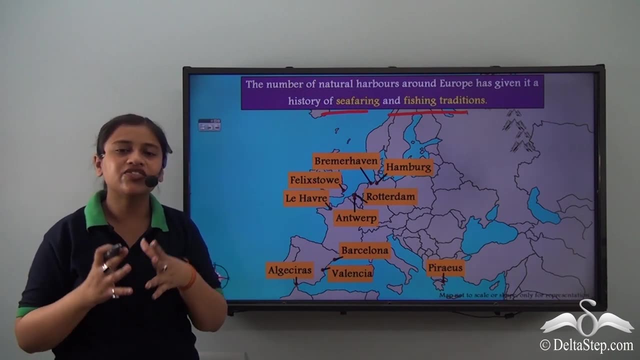 it a history of seafaring and fishing traditions, So sweden is one of the most important fishing fishing traditions. so we just learned that the indented coastline of Europe has given rise to many natural harbors. well, these natural harbors have proven to be very, very beneficial for the country. why? because they have a history. 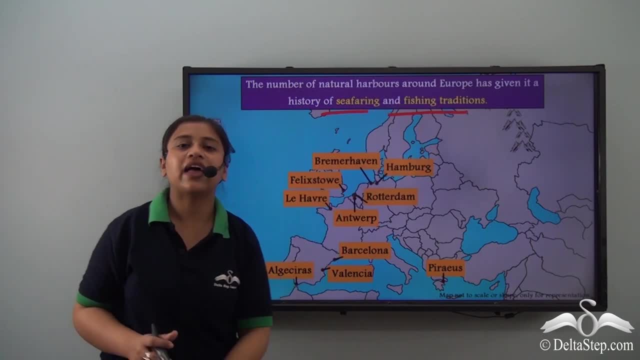 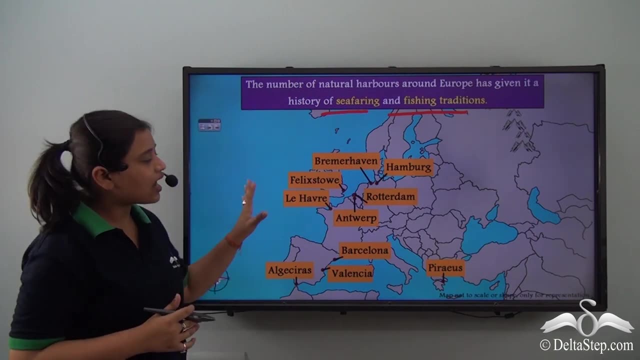 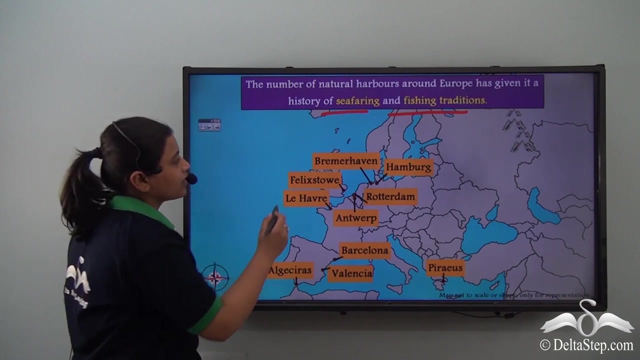 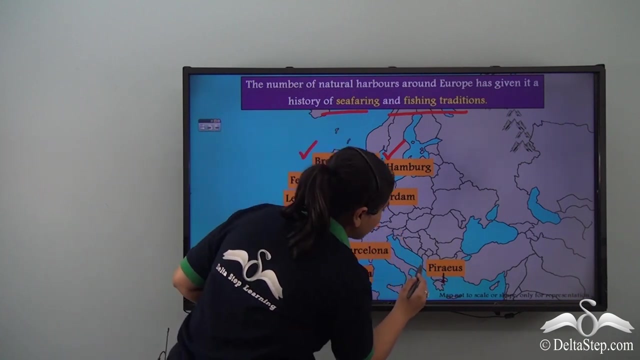 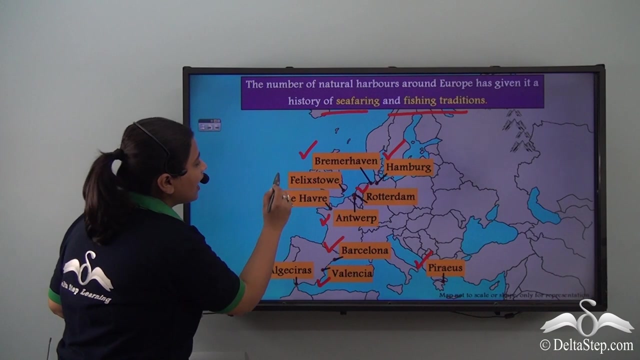 of seafaring and fishing traditions. that means that it has helped boost the economy of this particular continent. so the natural harbors of Europe are many, however, so the most important natural harbors are Bremerhaven, Hamburg, Rotterdam, Antwerp, Piraeus, Barcelona, Valencia, Algeciras, Le Havre and Felixstowe. 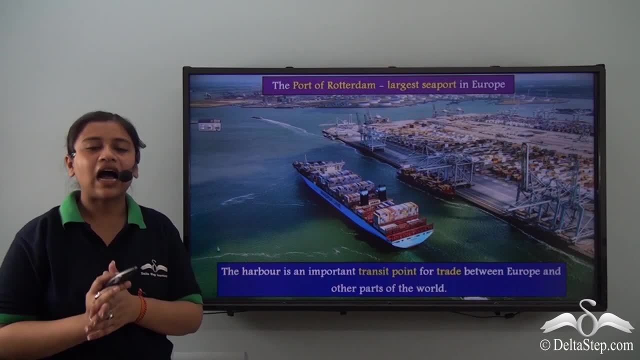 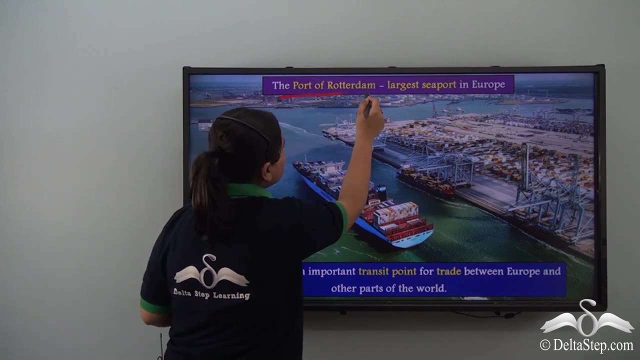 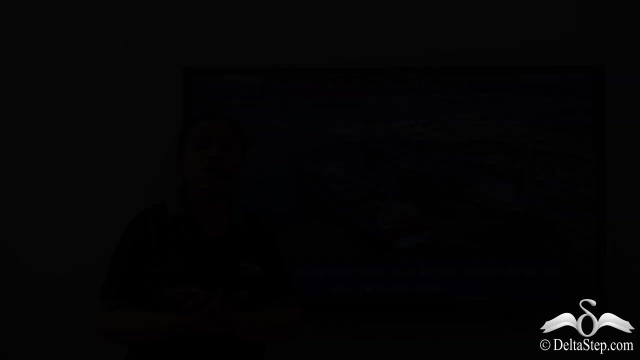 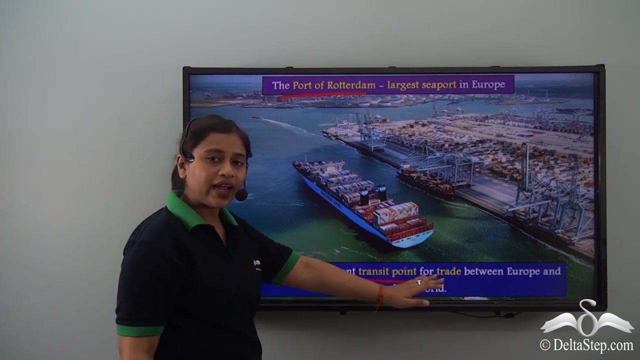 Out of all these natural harbors, the largest seaport in Europe is the Maritime Harbour. The port of Rotterdam is the largest seaport in Europe, and not only is it the largest seaport, it is also an important transit point for trade between Europe. 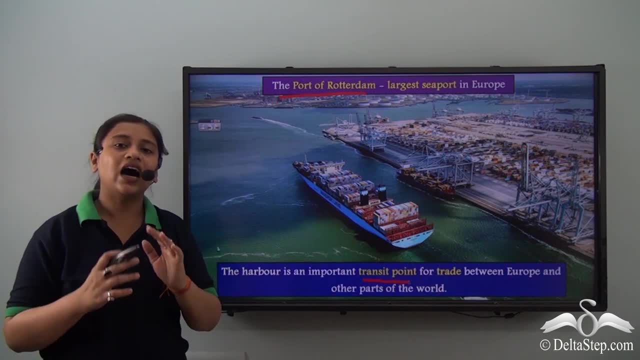 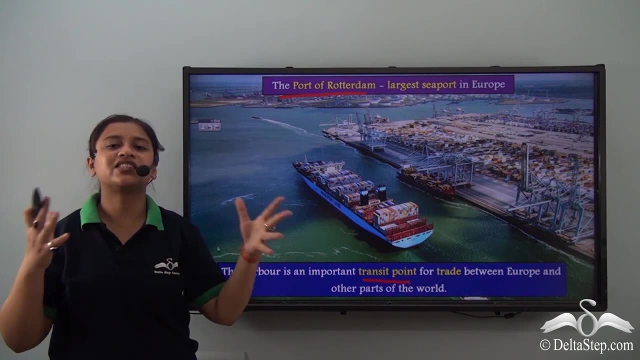 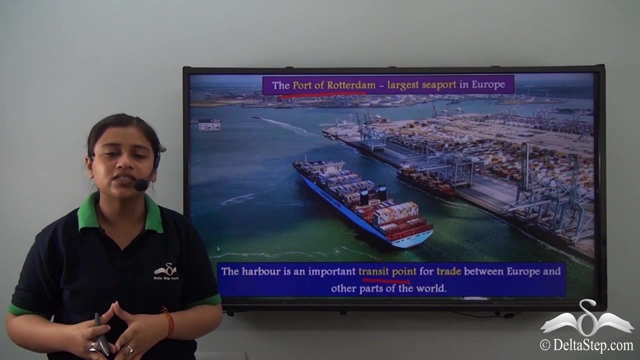 and other countries of the world right. other than that, this particular port is a very innovative port, as it has eventually expanded over the years, giving access to many hybrid ships. other than that, it has also committed to the goal of CO2 or carbon dioxide neutrality, so the history of seafaring can be dated back to the age of discovery. 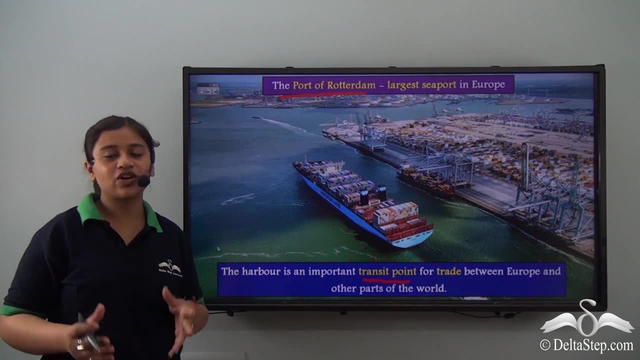 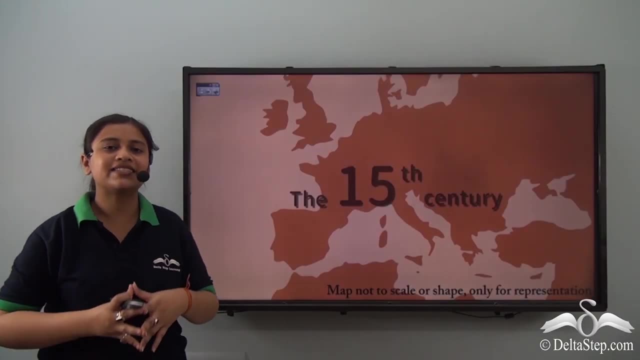 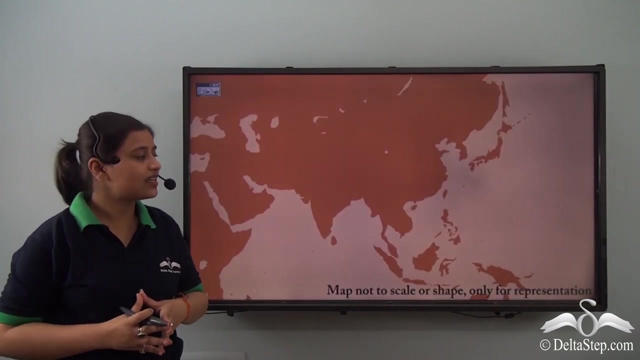 where Europe had a central position or a key role to play. so let's see how. so the age of discovery can be dated back to the 15th century and Europe was at its center. Europe that there were huge deposits of spices and gold on the eastern expanse of Asia. So it 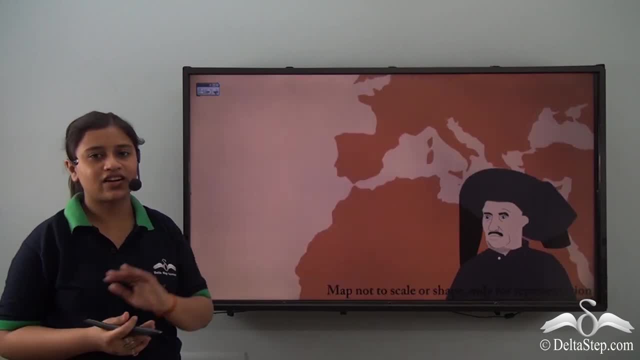 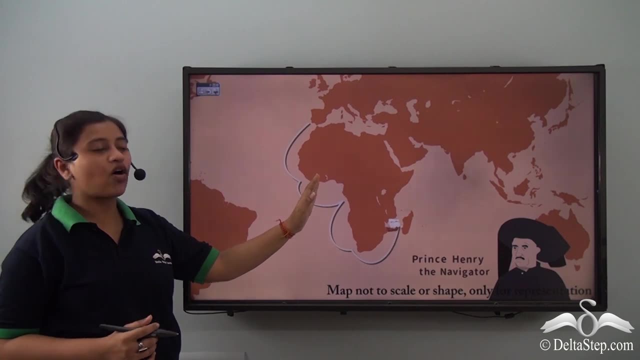 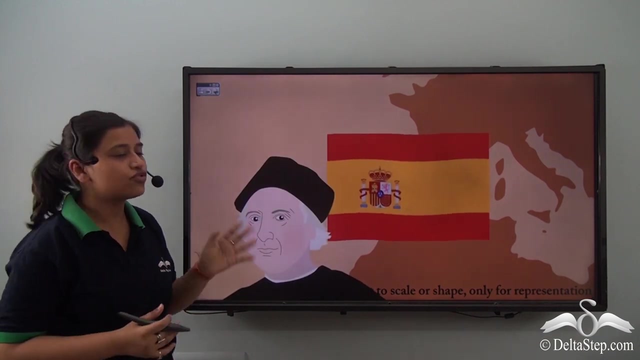 decided to take a direct route to these Asian countries. Portugal's prince, that is, Prince Henry the navigator, explored the western part of Africa and many explorers followed him. where Vasco da Gama actually found the direct route, to India, Spain was not ready to fall. 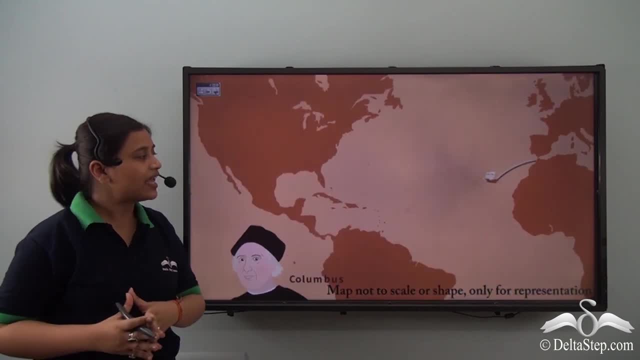 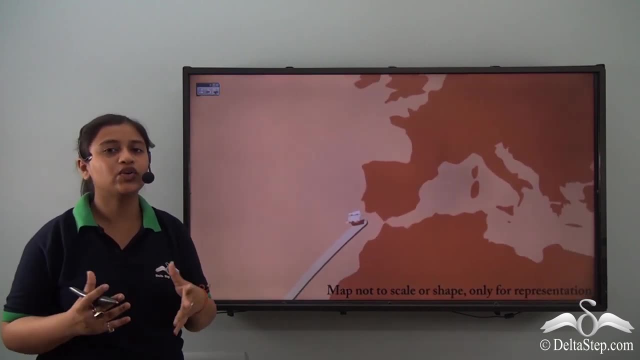 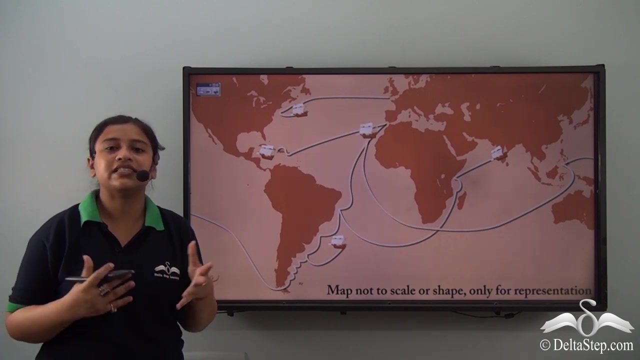 back, and so decided to do the opposite of Portugal. It went out to look for Asia by advancing towards the western side, where it ended up exploring the new world. However, when the sea routes or the art of sea navigation became very developed, many countries of Europe 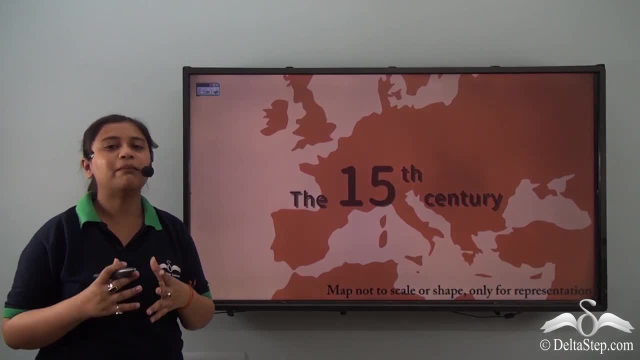 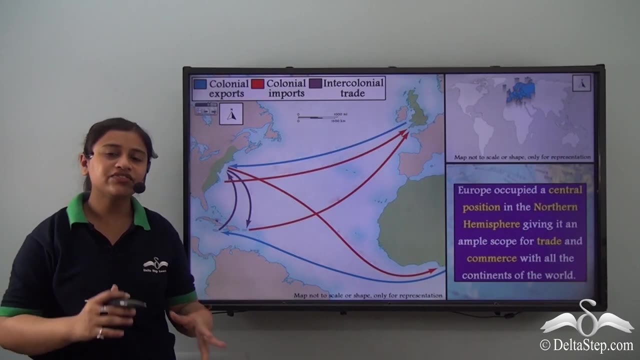 spread across the world and explored many parts of the world. So when the European countries explored different parts of the world, or the new world, they did not waste any time to spread its colonies across the world right. So on spreading its colonies, Europe not only expanded its 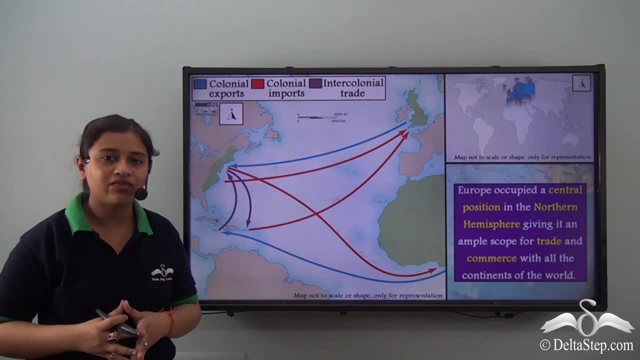 trade but became one of the most important powers or colonial powers in the world right? So you can see on this map that the red lines here. this indicates that Europe used to bring in or import raw materials from these colonized countries at a cheaper price and then manufacture. 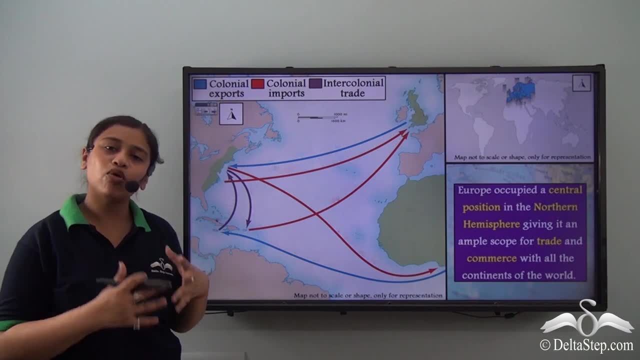 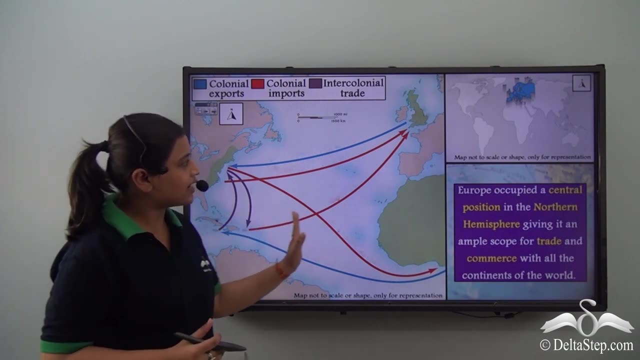 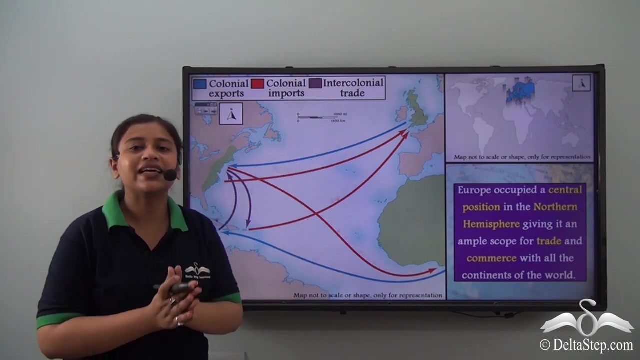 them using high technologies and then export these back to these colonized countries and sell it at a higher price. So, while these red lines indicate the colonial imports, these blue lines on the map actually show you the colonial exports, right Other than that, 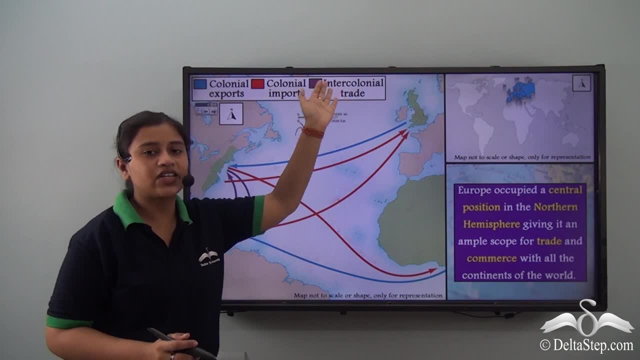 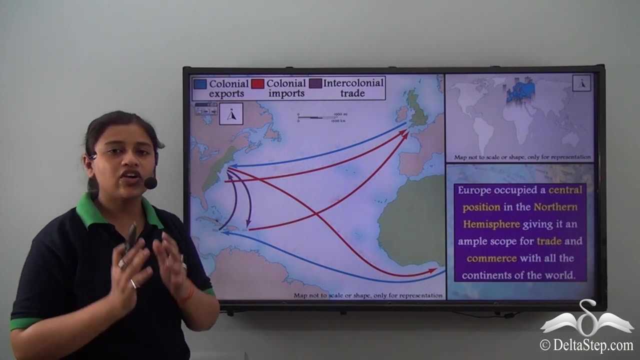 they were also the present of intercolonial trade which used to take place between the colonized countries. right, So you see that Europe, having a central position in the world, was able to carry on with its trade and commerce with all the countries of the 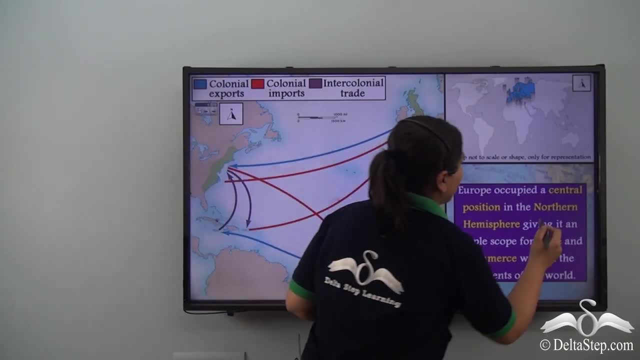 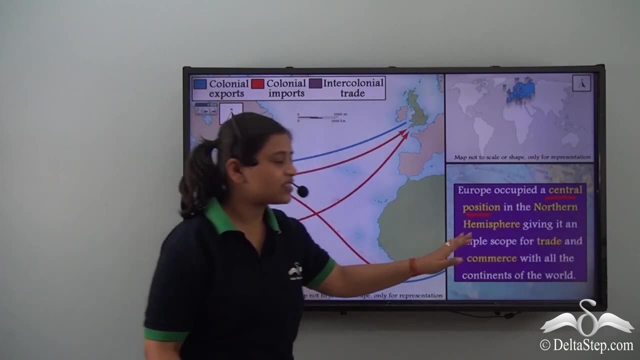 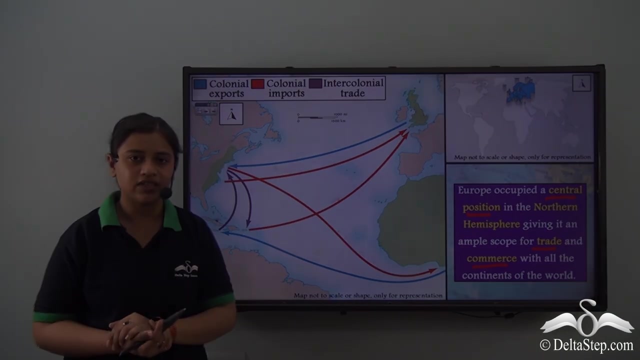 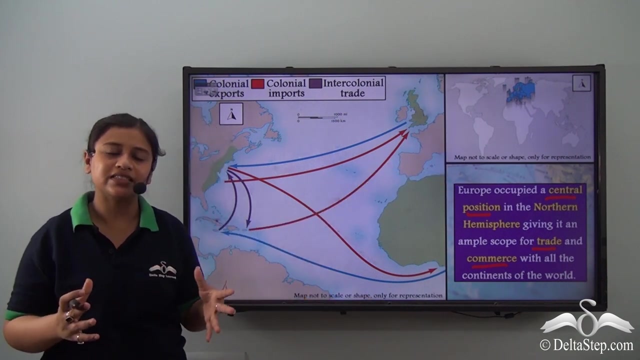 world. So we can say that Europe occupied a central position in the northern hemisphere particularly, and this gave it an ample scope for trade and commerce with all the continents of the world. So all these factors, be it its location, be it the natural harbors that were a gift of its indented, rugged coastline, so be. 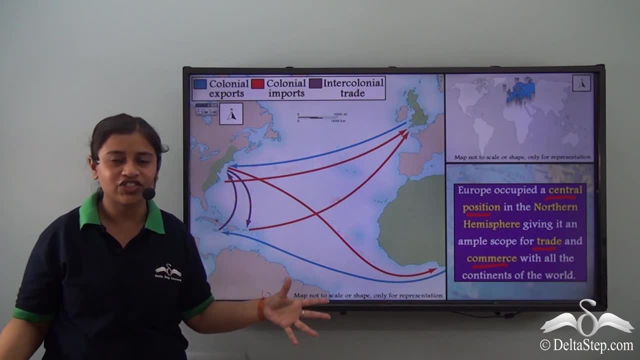 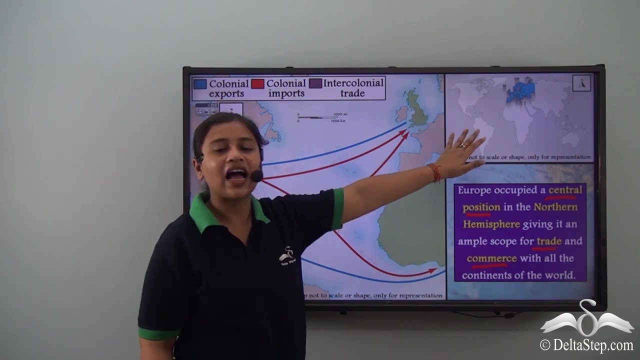 it a land of a great mythology, or be it a land which has been ruled by many kings and kings in Queens, with a diverse cultural heritage, or be it a land with many natural harbours that is a gift of its very rugged and indented coastline. Europe has been and is still a 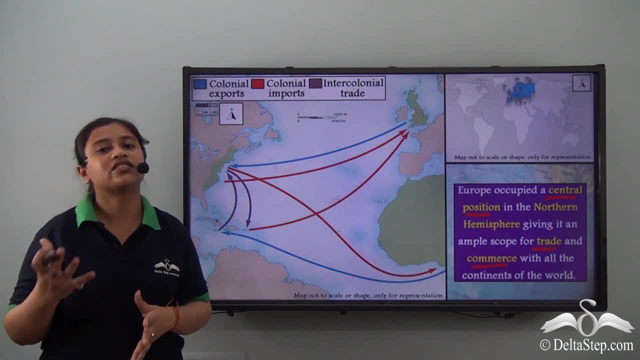 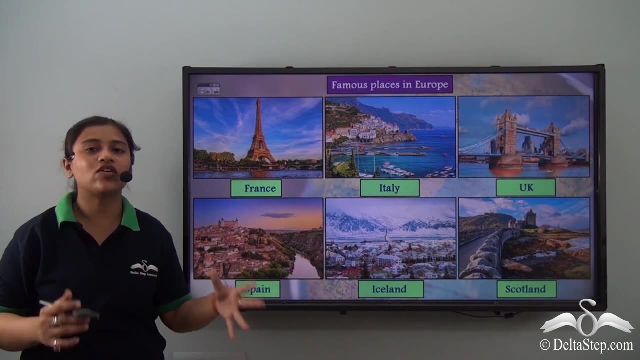 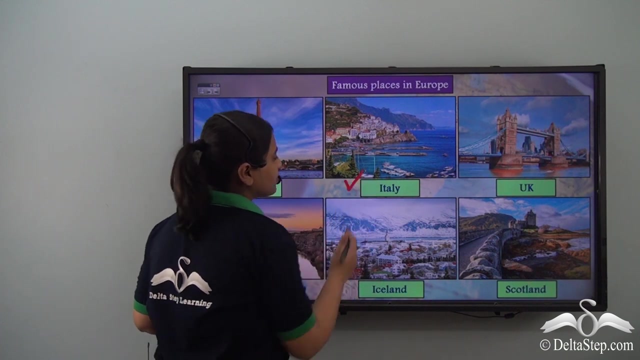 fascinating continent that attracts both researchers and travellers from across the world. So, besides being a fascinating continent in itself, there are various famous places in Europe. that makes it more attractive. And what are these famous places? We have Paris. in France, we have Italy. 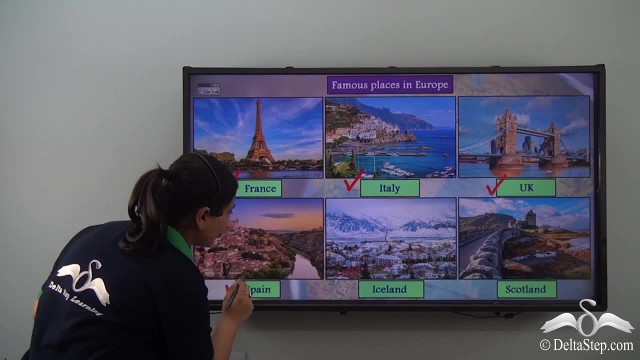 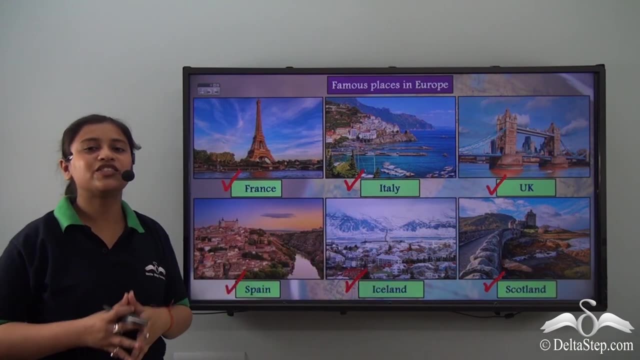 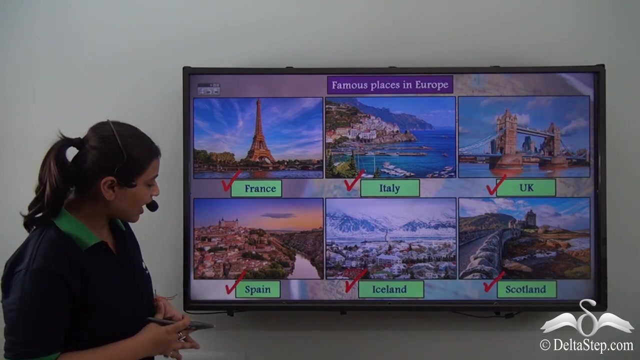 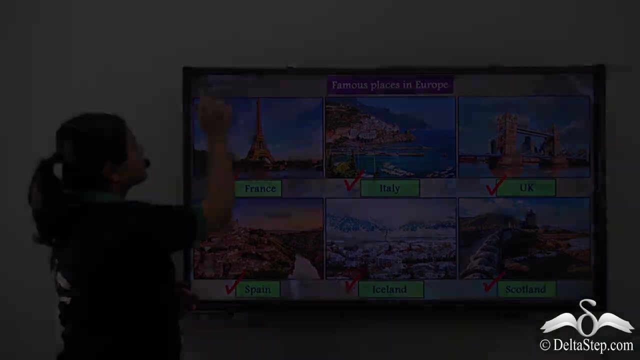 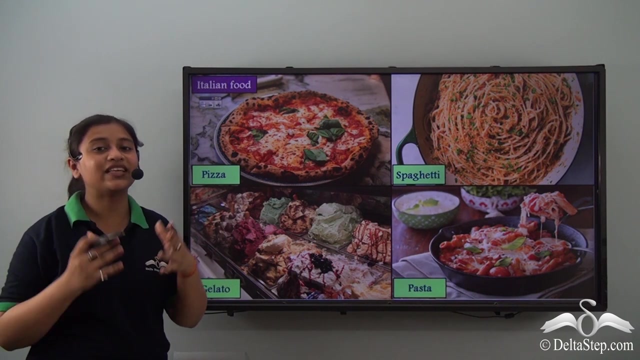 we have London. in UK, we have Spain, Iceland and Scotland. So, while France and UK are famous for their beautiful monuments, Italy is famous for its for its yummy, delicious foods. On the other hand, Spain, Iceland and Scotland are famous for its scenic beauty. Wow, the screen looks yummy. Well, we just now talked about the 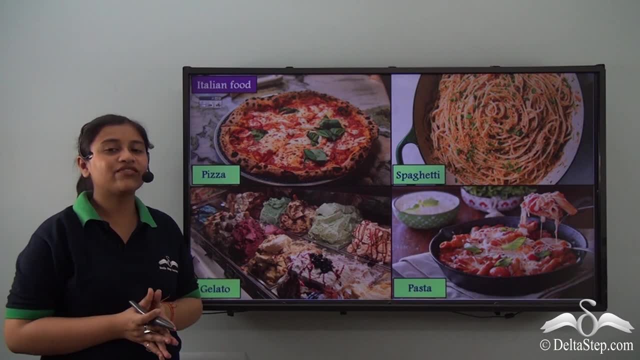 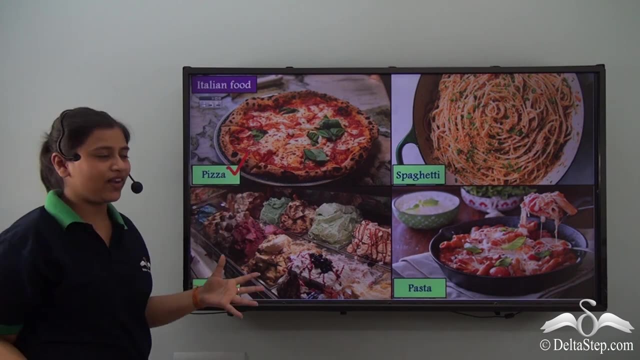 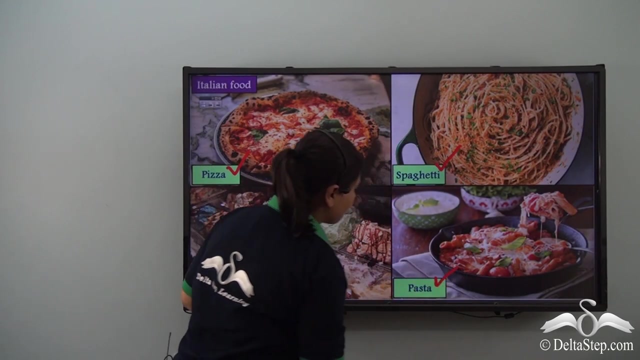 Italian food, the yummy Italian food. Let's see some of the most famous and most demanded chocolate foods. So we have pizza that we all love, then we have Spaghetti, then we have Gelato and we also have Pasta. So these are some of the most yummy, delicious food. 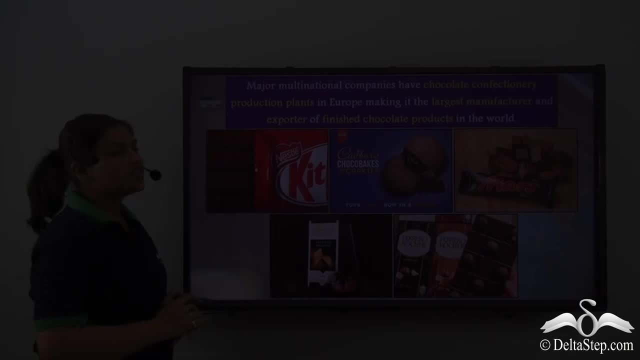 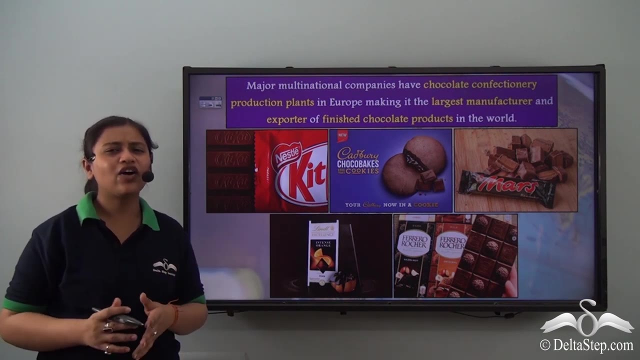 that you would never want to miss. So, while talking of food, we cannot really do away with chocolate. Chocolate is a favourite of so many people. Well, a huge production of this chocolate is a whole food with which we have to feed ourselves. So let's start. 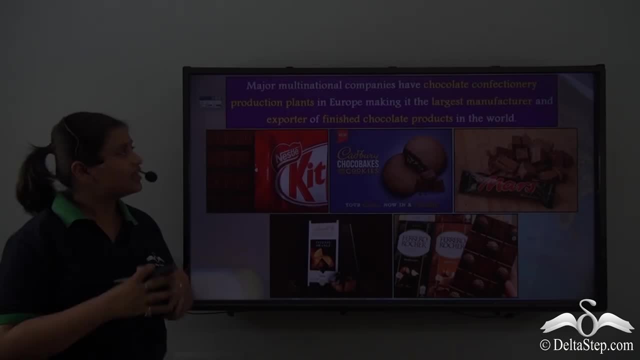 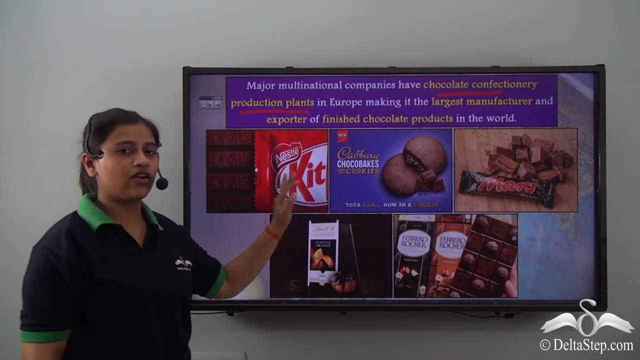 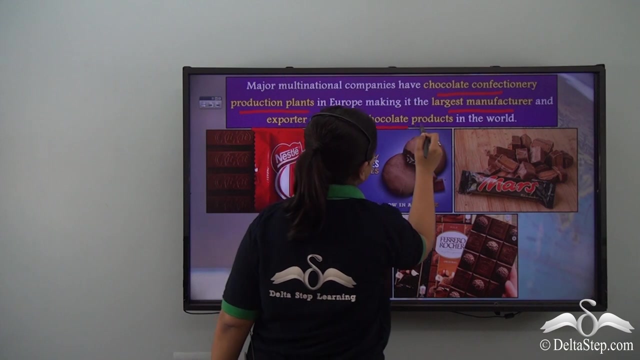 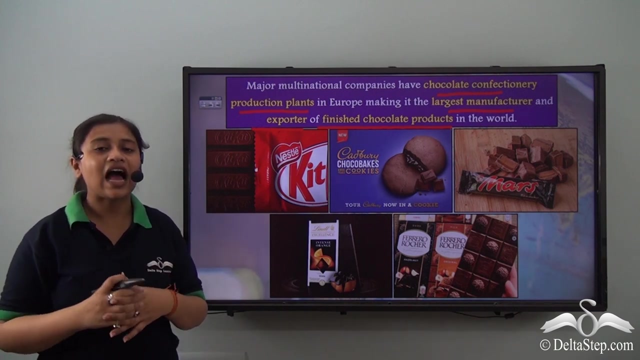 chocolate is done in Europe itself. The major multinational companies have chocolate confectionary production plants in Europe, making it the largest manufacturer and exporter of finished chocolate products in the world. So some of the major multinational companies of chocolate have their confectionary chocolate production plants in Europe, making it not only the largest 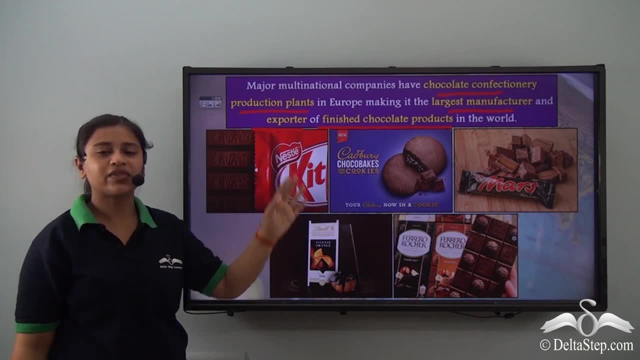 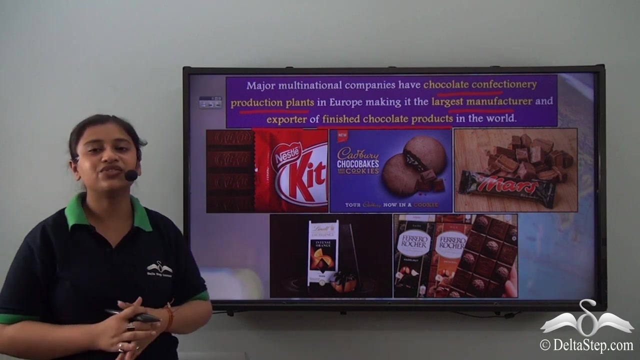 manufacturer, but also the largest exporter. By report of 2020, about 76 percent of the global chocolate sale was from Europe, So you see that some of the most delicious and most demanded chocolates are produced in Europe. So in this video, we learnt about Europe as. 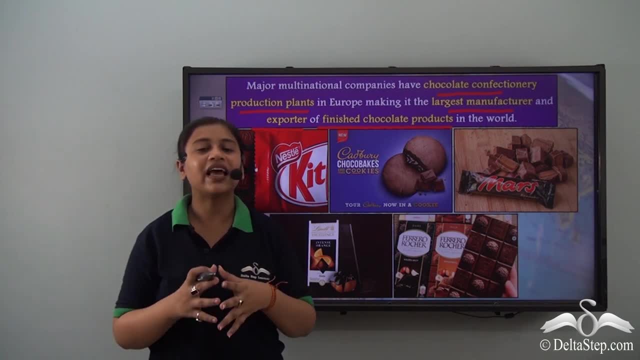 a continent. We understood that Europe has a central position in the world map right. It is not only an important power but a fascinating continent to visit. We further learned that Europe not only has a diverse and rich history, but we also learned that its rugged and indented coastline 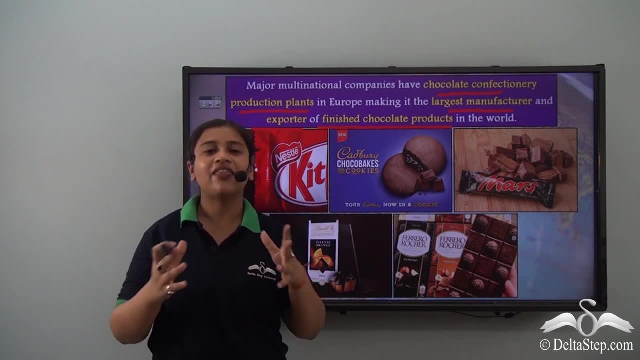 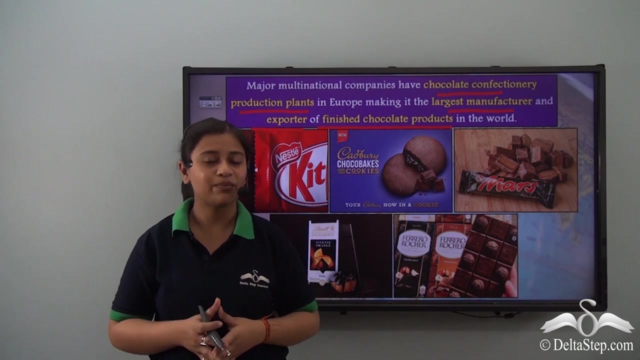 has gifted to it many natural harbours. that has helped boost the economy of Europe. So we see that Europe is a very interesting continent to learn about. In the next video we will be learning about the physical features of Europe in details. Don't forget to subscribe to our channel and hit the bell icon. 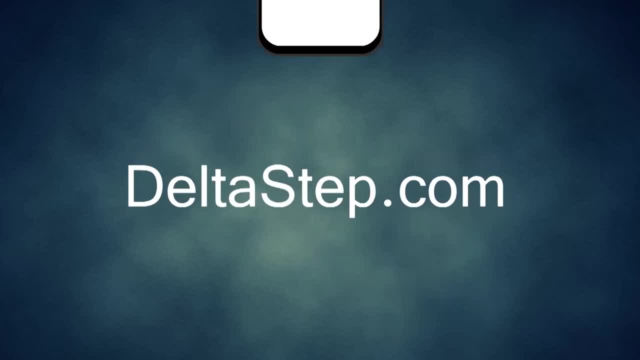 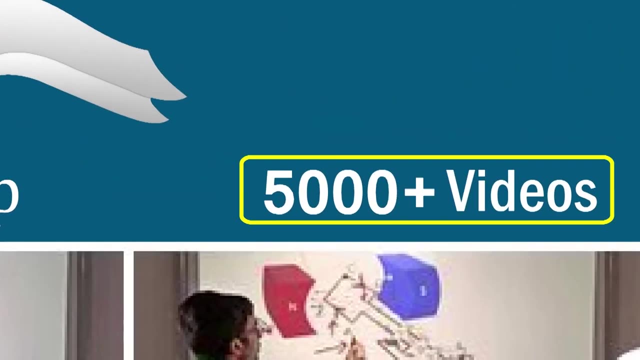 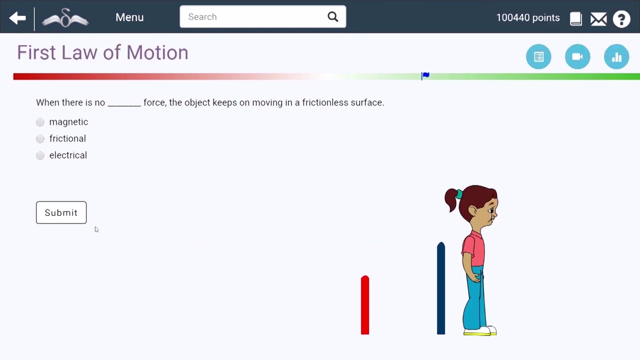 You can also register for free at deltastepcom or download the Delta Step app to learn one-to-one with our amazing teachers or to get access to all our 5000 plus amazing videos as per your school syllabus. Master each topic with our adaptive practice technology.